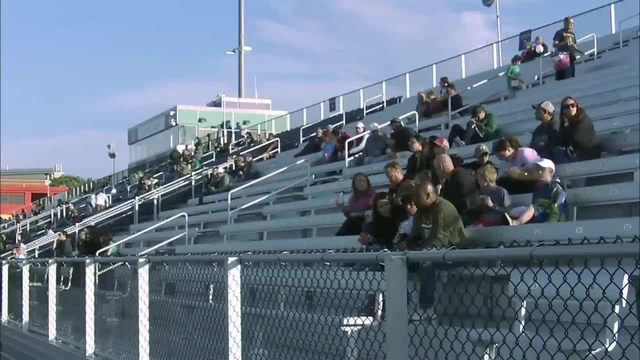 What's going on, guys? Welcome back to another game analysis video. In this game, my team, Hartford Athletic, are taking on Detroit City FC, And now I think this is my best performance ever as a center mid- And that's not saying a lot, because this is only my second game. 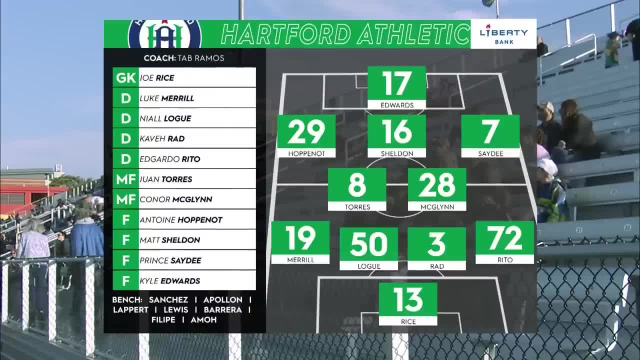 ever as a center mid in my professional career. So yeah, it's a new position for me. I've played like 140 games, I think, most of them at right back or left back, some at right winger, left winger and even some at center back, But this is the first time I've ever played in this central. 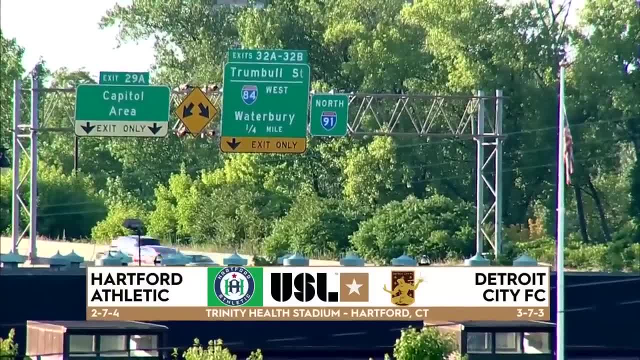 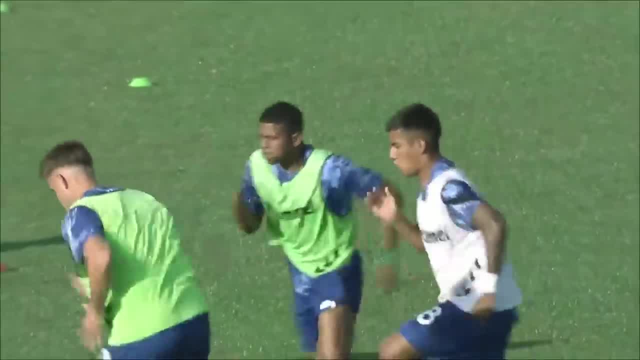 midfield position. Now, usually when it comes to these game analysis videos, a lot of it is kind of like me almost teaching a lot of you guys or you're watching like what's going through my head and, kind of honestly, an instructional video of how to play the position, And now this is kind 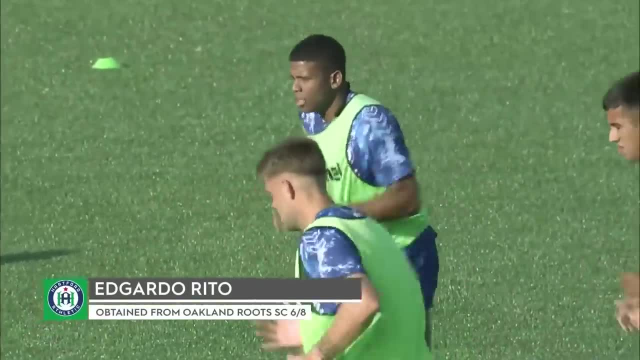 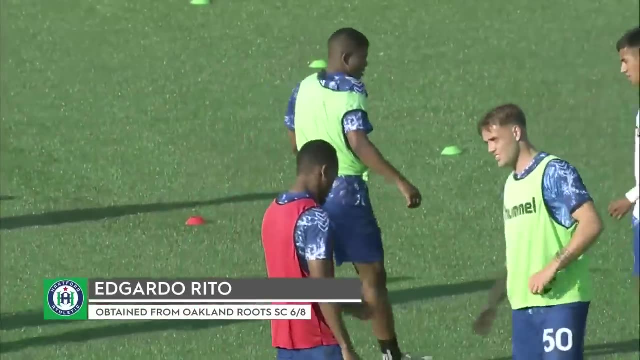 of shifting a little bit more to me learning the position and kind of learning along with you guys. Now, obviously I'm a pro footballer. I still know where every position needs to be: off ball movements, on ball movements. You know. that just kind of comes. 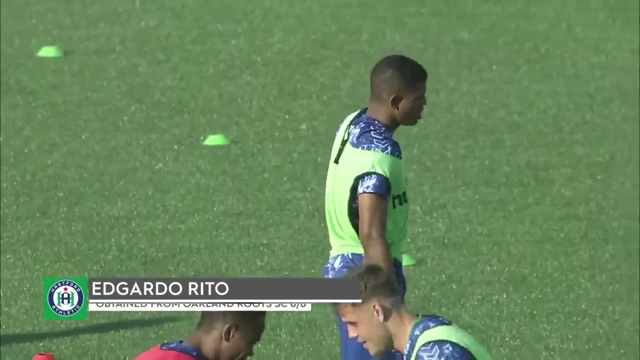 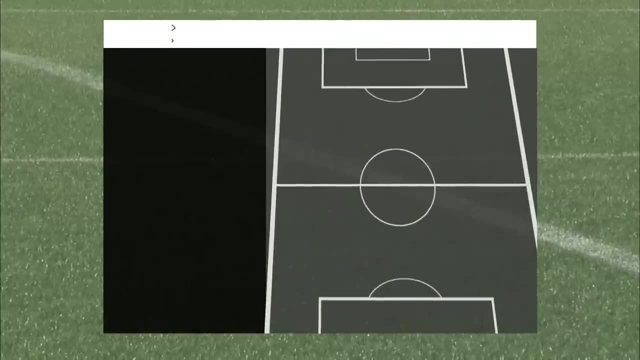 along with being a pro, but actually doing it in a professional environment is something completely different And I found- you know playing here, that the little things that I would take for granted as a right back, like knowing exactly what to do and just feeling so natural. 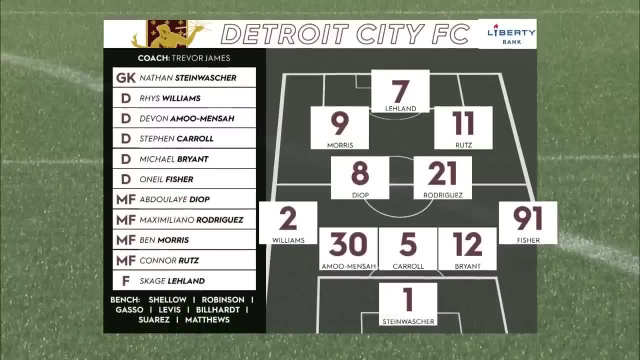 was very unnatural coming in here into that attacking center mid position. Here's the lineup for Detroit city. They're coming out with five in the back like a 5-2-2-1 or 5-4-1, whatever you want to call it. But yeah, let's just get into the video. 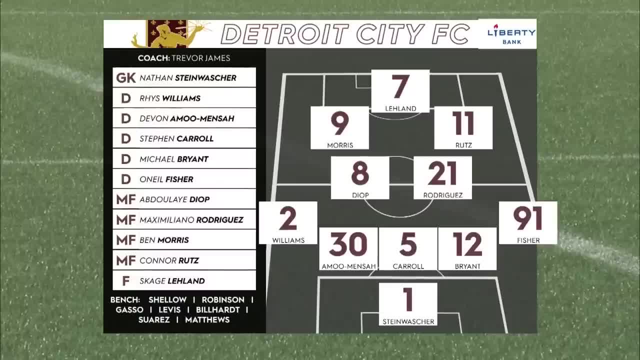 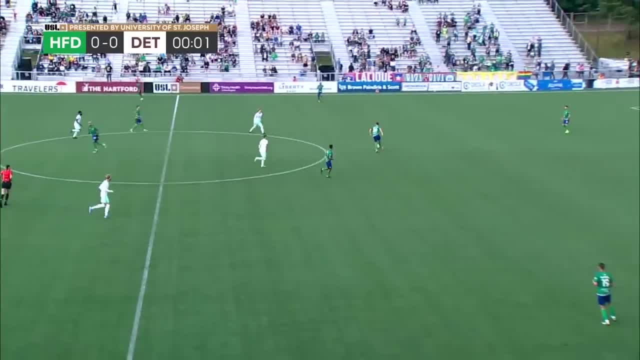 get into every touch, Get into my analysis and uh, and you guys can see how I played this attacking center mid role. So we're going to start off with the kick. We are the green and blue team. Detroit city is coming out in the white and looks like like mint green colorway. Here's my very first touch in the game. 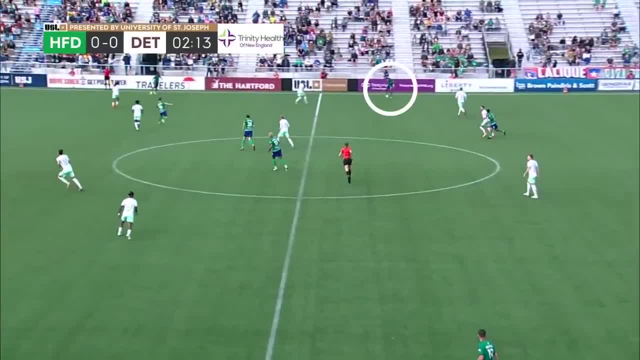 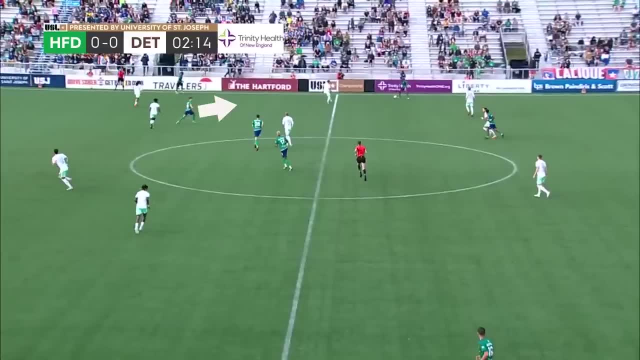 coming up. after this right here ball comes into my right back immediately. I'm just kind of doing what I would want my center mid to do in this position If I'm playing right back, which is check away and then pop into this space. So you can see my first movement to my left and then I'm 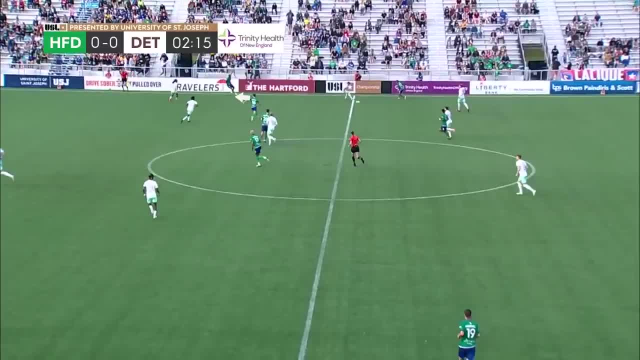 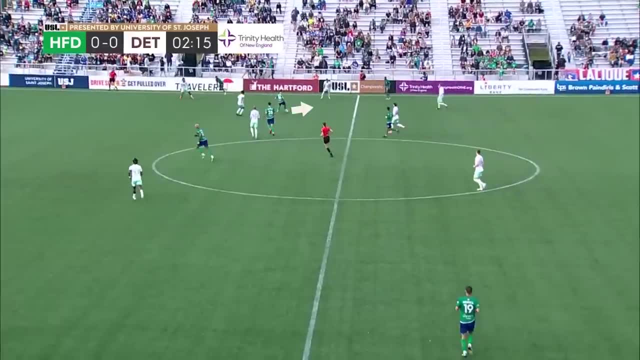 going to pop right in here between all these players. I'm checking my shoulder, looking forward see if I can hit this ball down the line. I'm seeing a lot of pressure come in, So I'm going to take my touch away from that pressure with the outside of my right foot back into space. 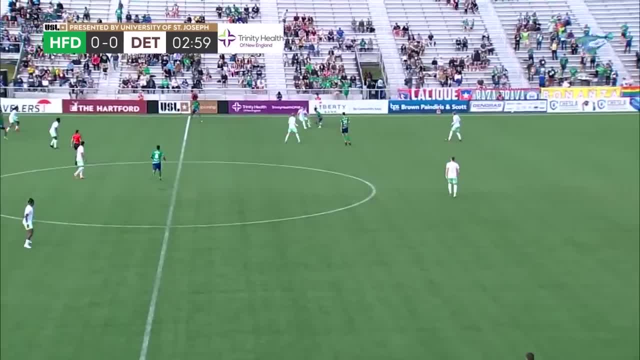 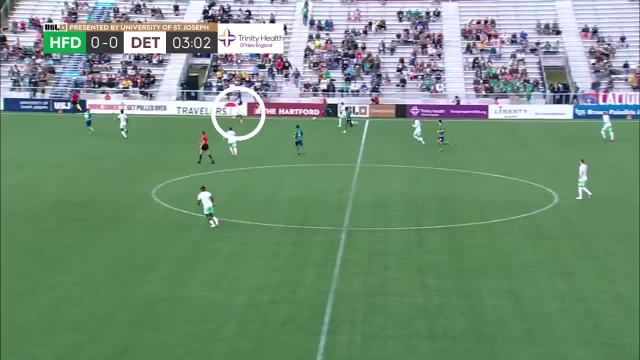 drive a little bit and then play back to my center back, just so we can keep the ball right here. Now, once again, ball comes into my right back. Now instead- you can see I'm kind of in front of my guy- this left wing back really steps here, So I'm pointing, I want the ball down into. 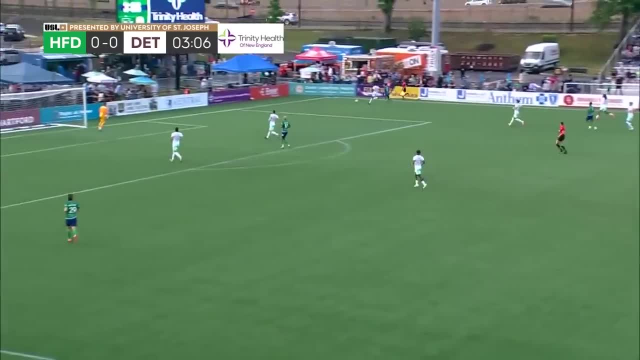 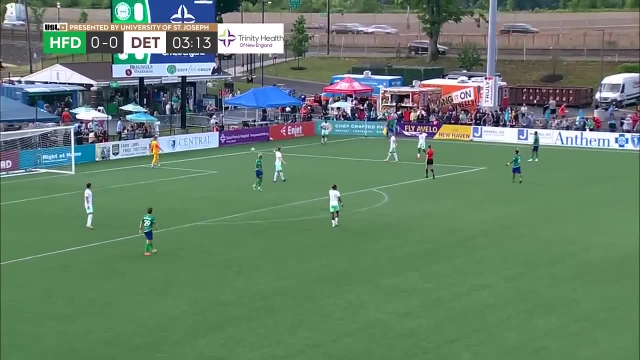 space. It's a great ball in. I try to control it, mistouch it a little bit And then it just goes out, push their defender into the ball And I don't even actually think he touches it. but they call a corner kick here, which was a kind of fortunate turn of events for. 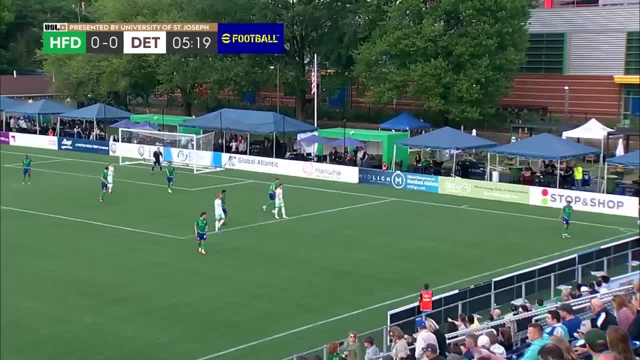 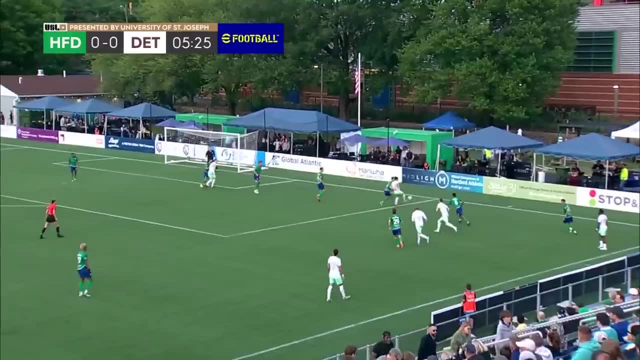 us So end up getting the corner kick here in the fourth minute. Now, defensively, here's my first action in the game. I'm off the screen. I was going to follow in Maxi Rodriguez as he makes this run in and then apply a lot of pressure. I really don't want to give up a foul here because. 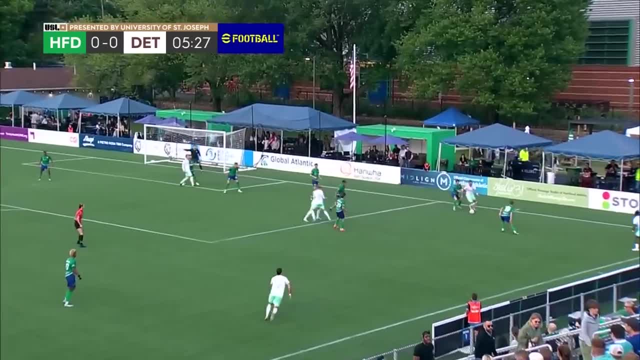 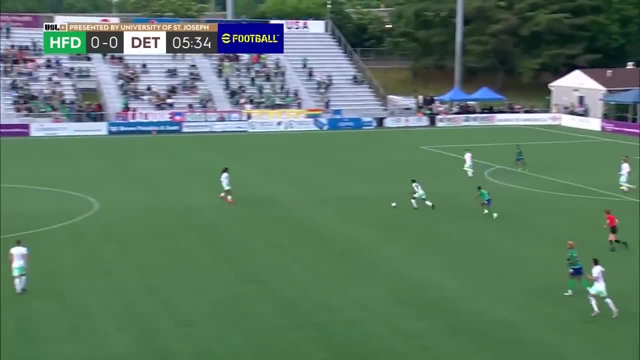 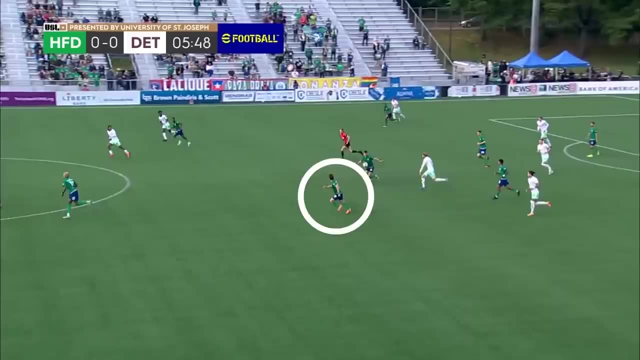 it could be inside the box for a penalty, but just even generally, this is a really dangerous area to lose a concede, a free kick there. So I'm just applying a lot of pressure but not giving myself away and and fouling here Now, right here. this is my first mistake. This is great one too, Antoine. 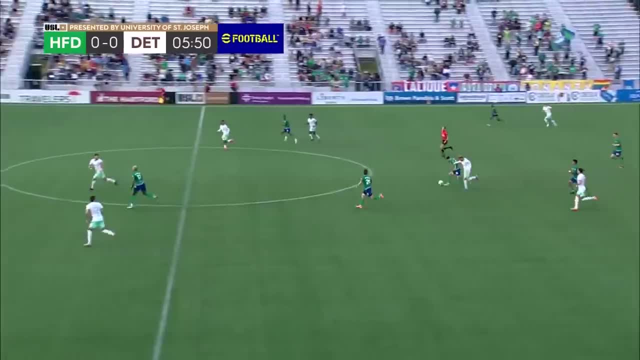 plays me the ball. He wants the ball back. He's got tons of time and space. It's not bad to drive in, but look at him, He's wide open. If I would've played this ball here, it could be a three V three. 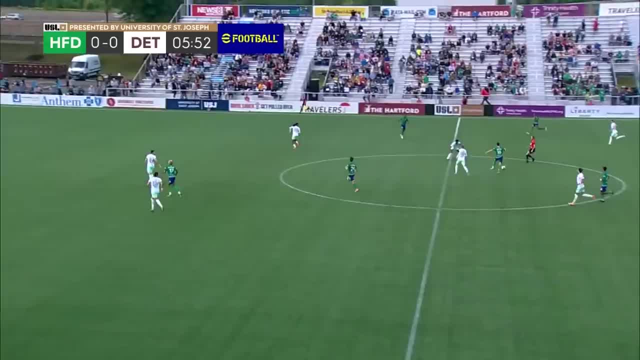 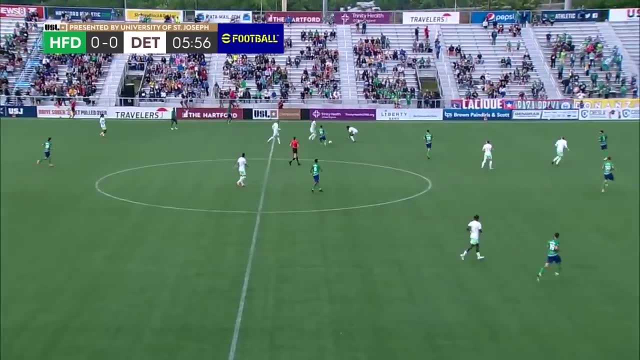 counter attack. Instead, I keep on driving a little bit and then I should. I'm looking for Prince here. I should just play Rito. I'd take another, you know touch. It's way too many touches here. I need to simplify it here and just and just play, play into Antoine, so he can. 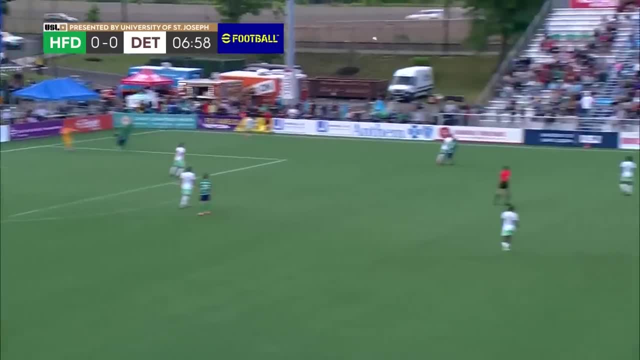 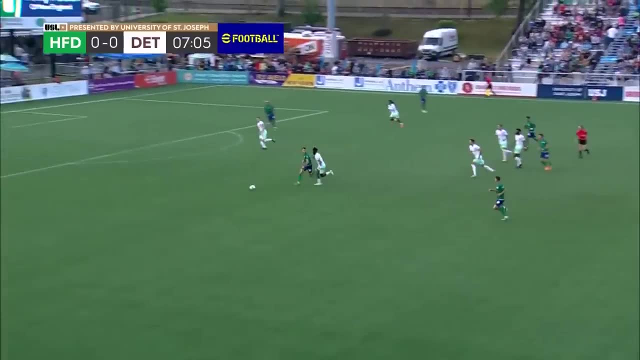 take the ball, Or if I don't see that and I take my touch out to the right play into Rito, my right back. So doing a little bit too much there and lost the ball because of it. Now trying to bring the ball down here, get a little bit lucky with that ricochet, but now the ball kind of kind of. 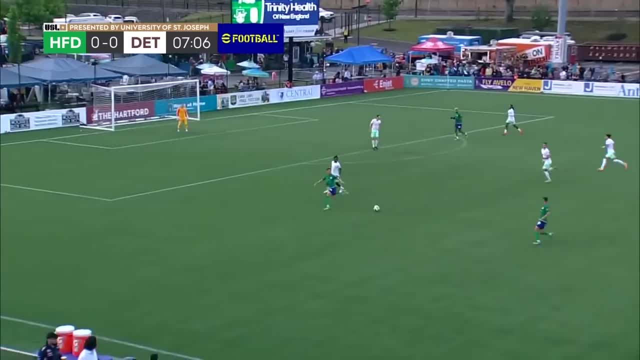 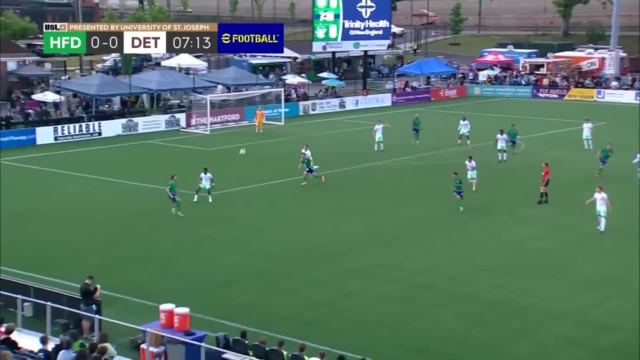 kind of goes in behind Detroit's defense. I know this defender is going to get back in time. I'm just going to play back into my left back and stay wide. Luke tries to find in Kyle Edwards our striker, and then the ball bounces back to me. 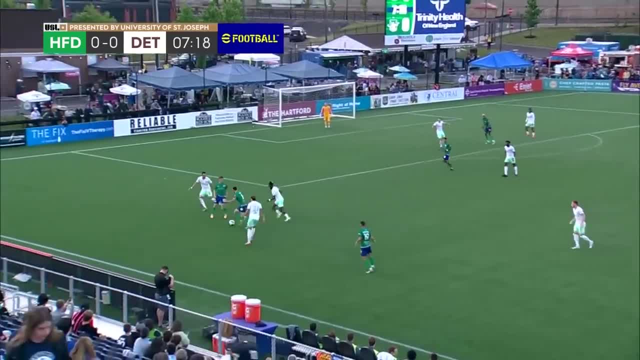 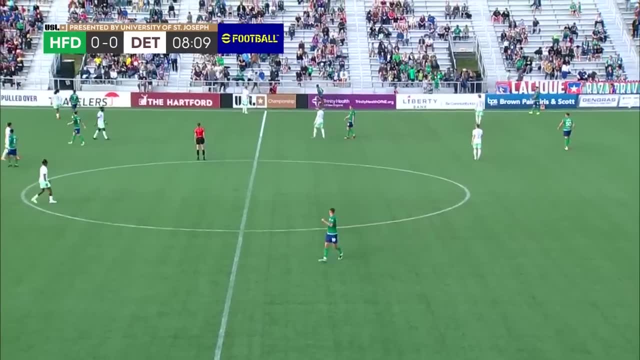 Drive inside a little bit, uh, keep possession of the ball here. And then, as I kind of drive down the sideline, it's getting way too crowded, So I'm going to play the ball back to my left, back again, and we can circulate the ball once again. but a good job, We keep possession in that, uh, in their. 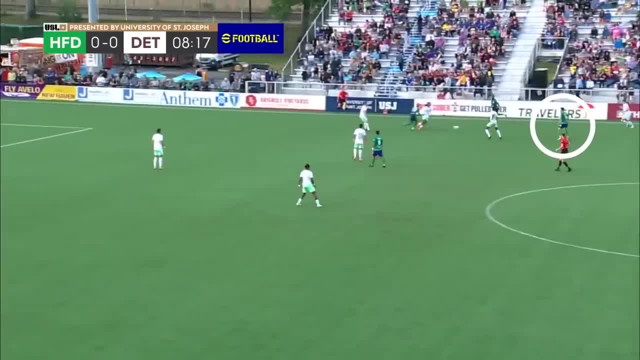 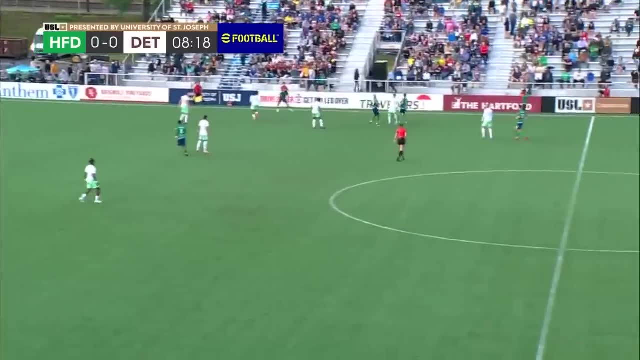 half, which at times it didn't look like I was going to do. um, ball comes right into our striker Elvis. It pops right back to me first touch. Now I'm just going to play into my winger Prince. It's kind of hard to see since it's over on the far side of the field, but he plays it back to. 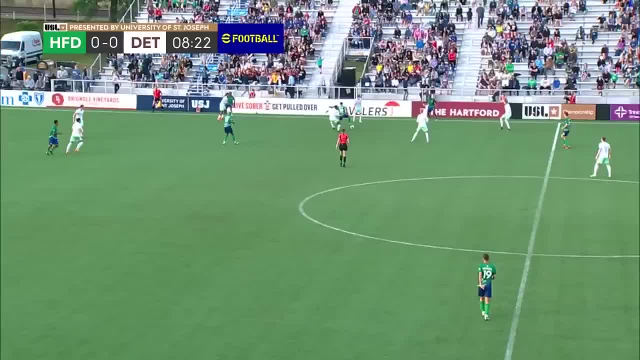 our right back, Who plays it back to me? And then I know I've checked my shoulder, I know I have a lot of pressure coming, So I'm keeping that ball away from this defender and just holding it underneath my foot And, as I feel, 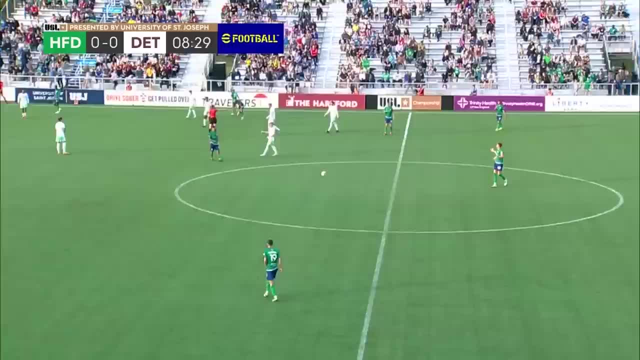 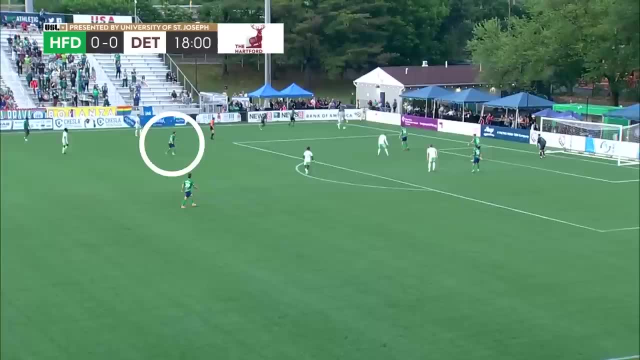 that contact. come in on my left side falling down and winning the free kick there. now ball in our own half. it's just kind of in the corner here. I'm just watching my guys starting to notice that we're about to get broken down, And then I'm just tracking back inside of the 18 yard box just to. 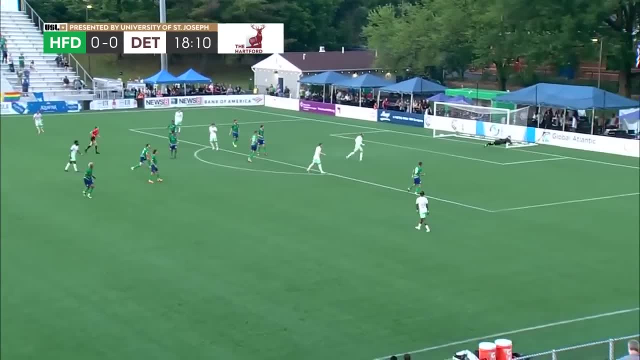 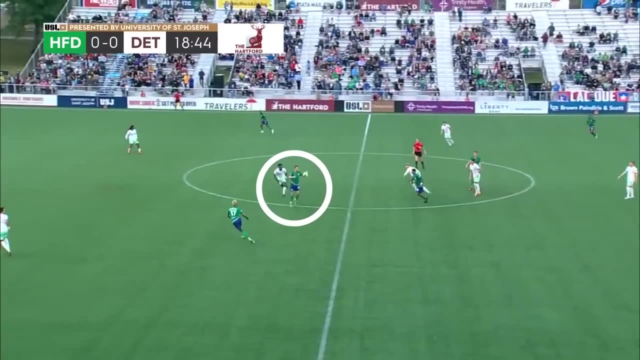 uh, just to protect that area, And then, just making my body big trying to get something in front of it, It bounces or ricochets off my heel here. Um, just to not make that shot an easy one, ball comes into. 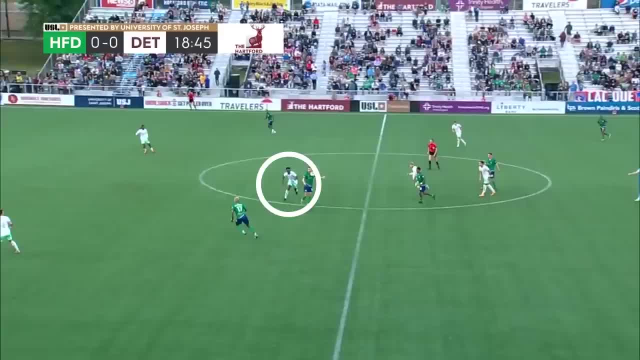 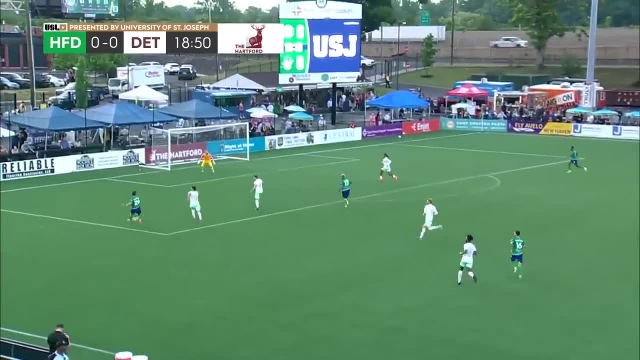 me. I'm looking at Kyle, I'm checking my shoulder. I noticed that this guy's right on my back So I can kind of take my touch with my right into that space, drive forward and then immediately play into Antoine and behind. I kind of had in the back of my head that I was taking a few too many. 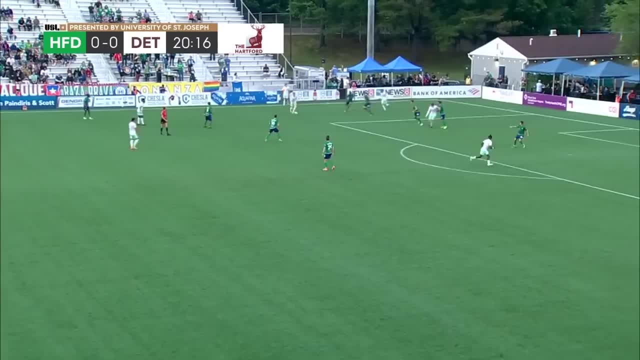 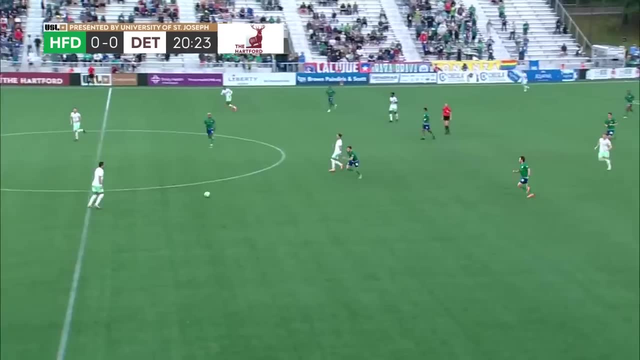 touches and driving a little bit too much and not releasing that pass quick enough. So on that play I was like, as soon as you beat the defender, play that ball in behind. I think that's a good pass. And then here this is defensively What. 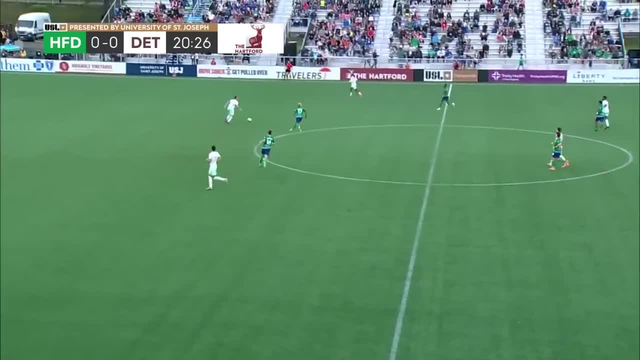 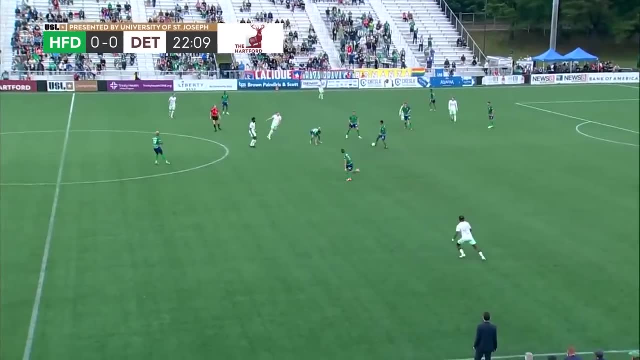 My coaches wanted from me: um, just because I have a little bit of a an engine, you know I can run a lot. So they just want a lot of defensive pressure here, making them try to play backwards and just making it difficult for those guys in the center winning possession. 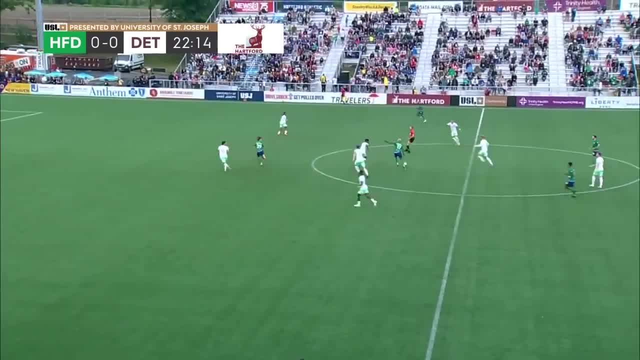 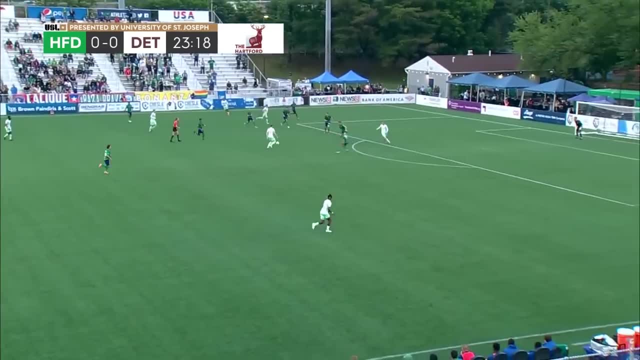 the ball there with a tackle- Um, it's a good counter attack. And then we ended up getting the ball out wide to uh, to Prince, to go down, Um, or I think it might've been out of bounds there. Now, next play ball comes in the center of the field and this is how they get their first. 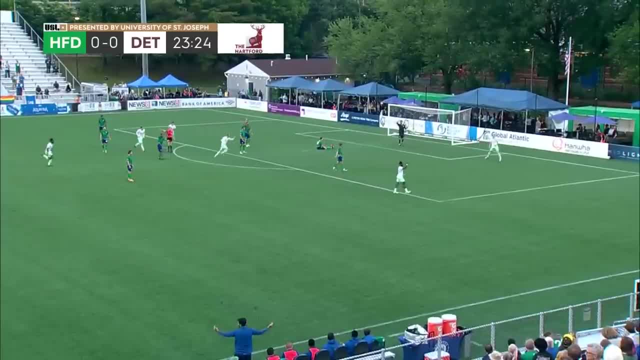 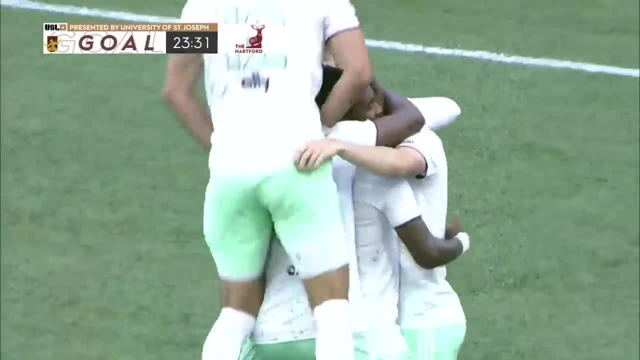 goal. It's a nice little one: two gray off ball movement And uh away the goal in the 24th minute And I just unfortunate- here I think there's a little bit of a miscommunication. It happens one player steps or two player steps um at the same time. 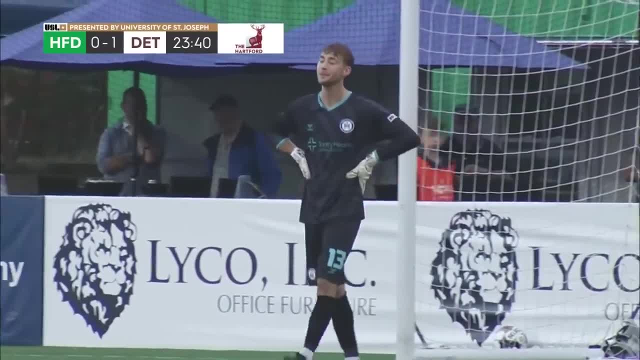 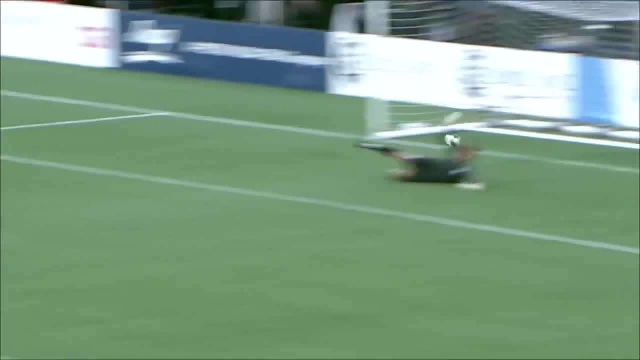 And it's hard to communicate that early on. but credit to Detroit. It's a really good goal And, uh, it's hard to defend. You can see here in the replay: just ball goes in behind because kind of shields his, uh, his man- I think that's Luke- shields Luke. 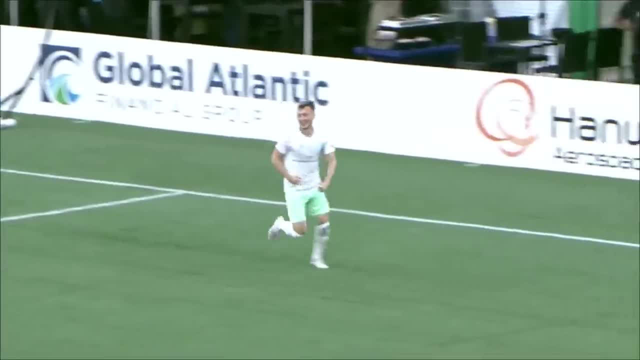 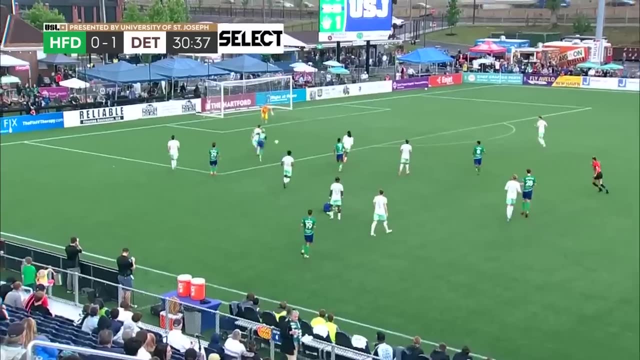 And then it's able to have this guy kind of run in behind and behind our defense and slot that, And behind it was next touch in the game falls up, just winning that header. And then I just get cracked on the side of my head, Um, after I win that header just hurt, Uh, but luckily. 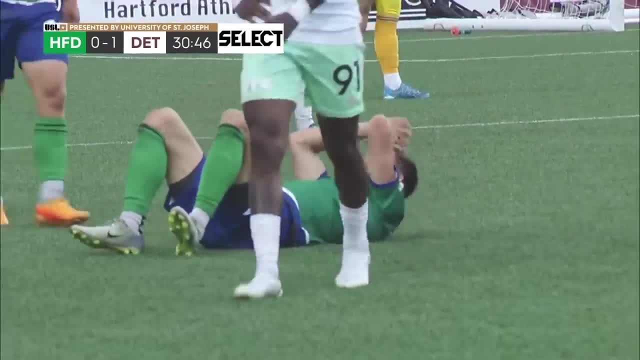 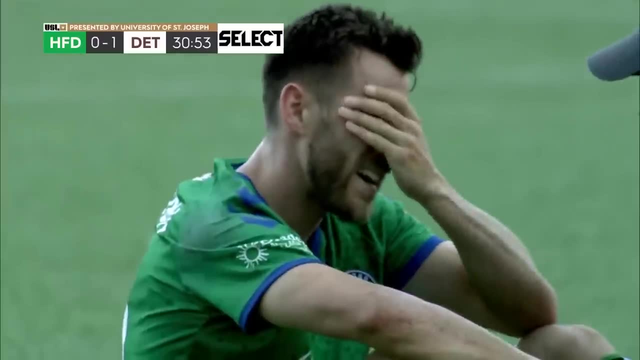 no concussion symptoms at all. I got tested. Our trainer comes over, does the full concussion protocol, concussion test tracks. My eyes ask me all those questions and everything, and I'm all good. So even though it hurt a little bit, I was pretty lucky with uh. 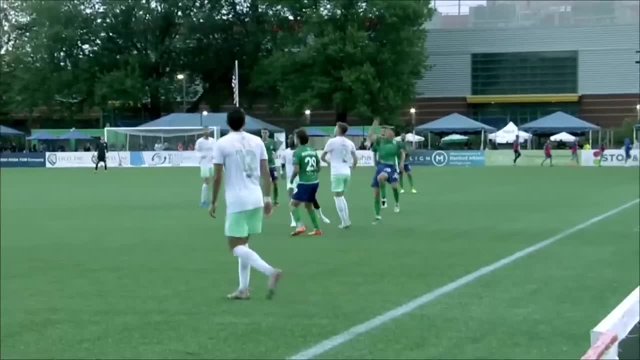 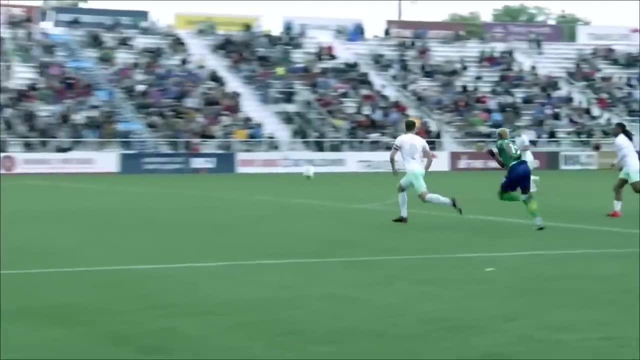 no concussion signs at all. And here's the replay that you can see: Uh just go up when the ball hits the header and then just heads collide right As I'm trying to flick that on, uh to Elvis. And now, this is why you have to be really, really careful with all the concussion protocols. 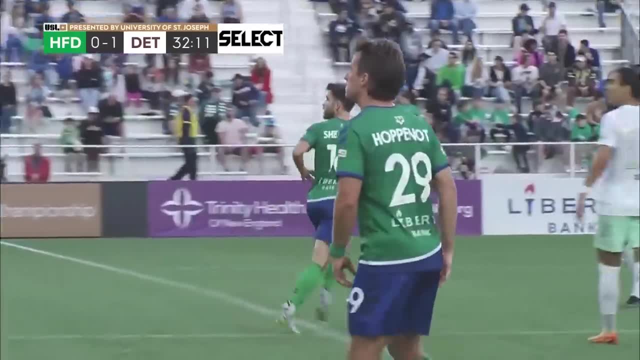 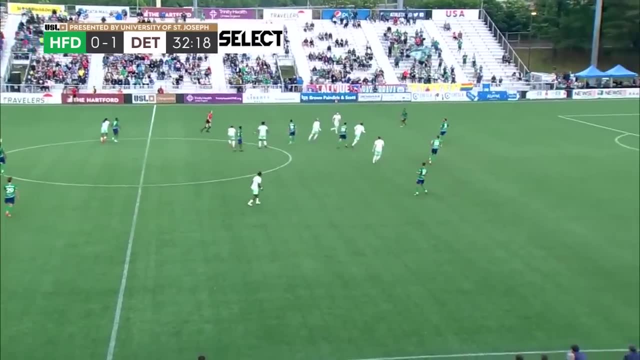 and take this seriously, Because as soon as I get back on the field, I step back on, I get cleared by the referees long ball from- I think it's a goal kick from uh Detroit- And I'm immediately have to go up for a header and win that header. And if, if, I would have actually had a concussion. 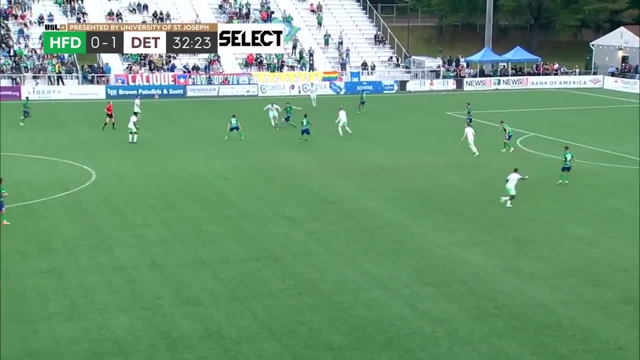 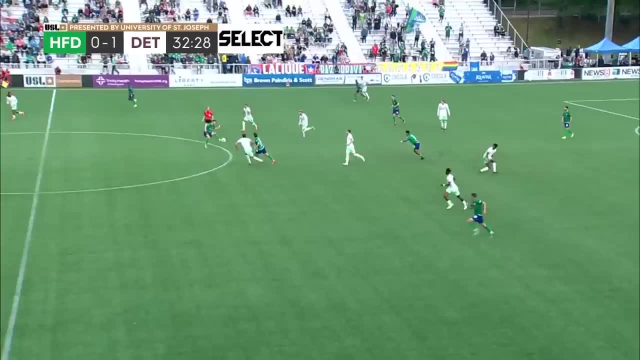 that would be really, really dangerous to go up for that and and sacrifice my head like that. Um, but good defense from us, Counter break comes right into me. And again, this is just me being. you know, I feel a little. 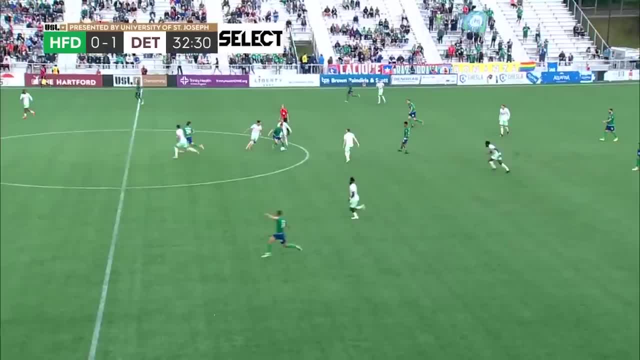 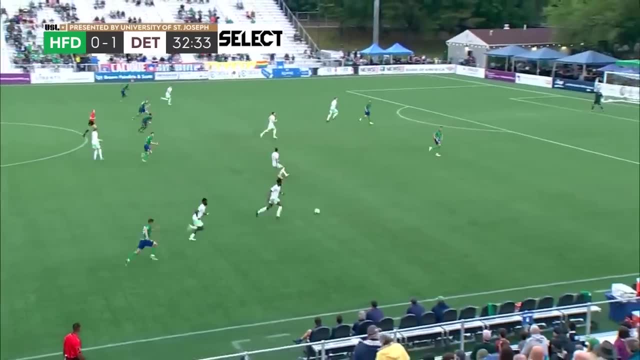 bit unnatural here and not recognizing this. receiving the ball, I do a good job to bring it down, escape that first round of pressure, but having guys all around me I miss it. Luke's wide open right here And I don't play that. I take too many touches. 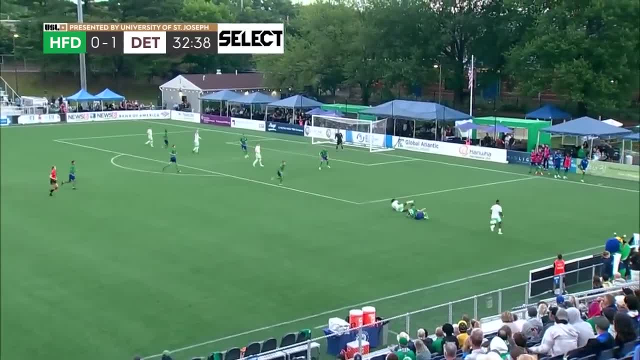 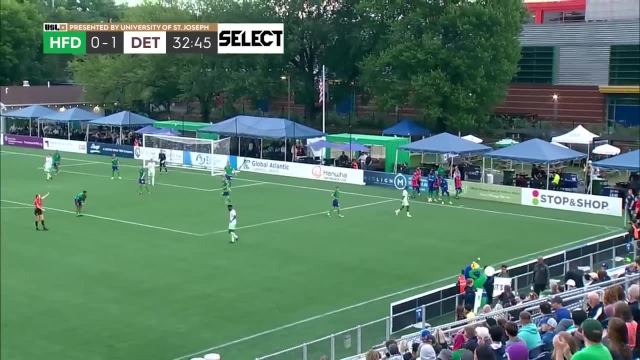 Just I'm used to having a lot more time on the on the wings. on the side of the field there's a right back And as a center mid- as as many of you guys who are probably playing center mid know- that you have pressure coming from the front, from the side, from the back, and you have 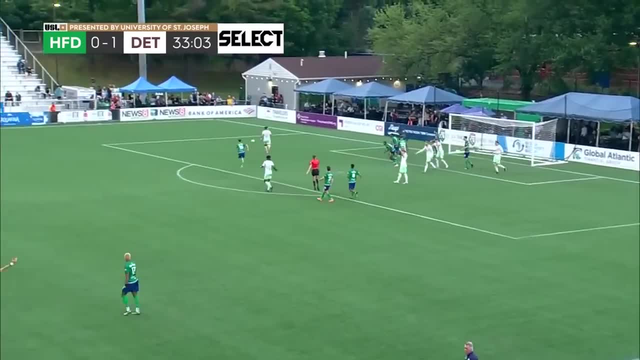 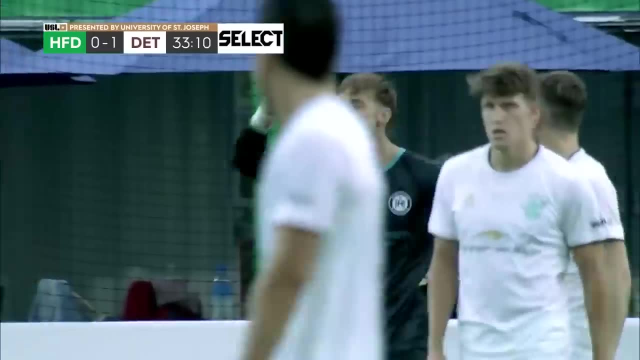 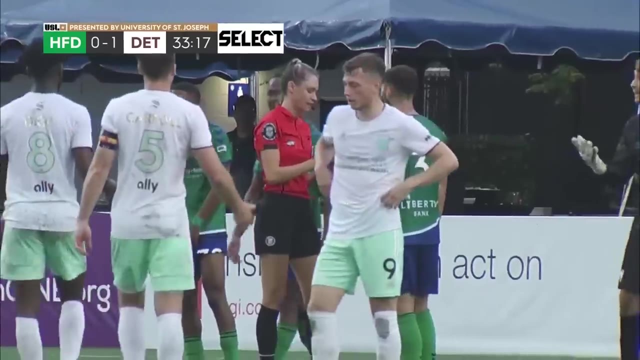 time to take touches as a center, mid and as a right back who's seen the whole field and usually only have one winger that you have to beat. Now, unfortunately, here we get a penalty called- I think it was on Prince Sadie- Our right winger just kind of brings down um one of the Detroit. 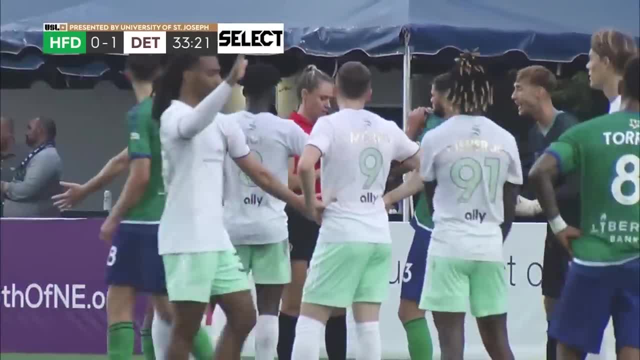 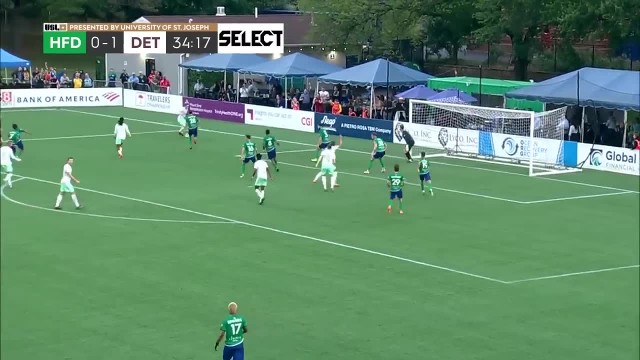 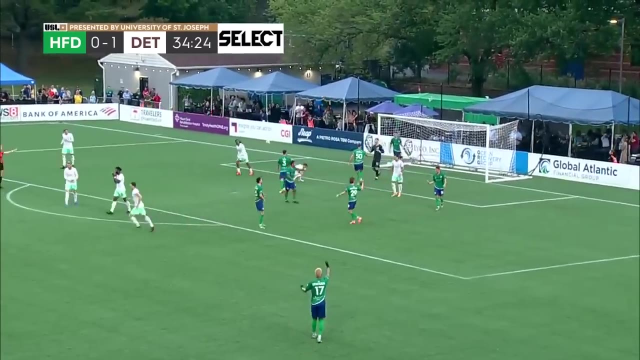 FC players as that ball gets crossed in the box. So not not. the best start from us here is the penalty from Detroit. Max Rodriguez, I think it's a pretty well hit penalty. It's right at that like. but Joe Rice, our goalkeeper, makes a great save and we're able to defend that, And, uh, they don't. 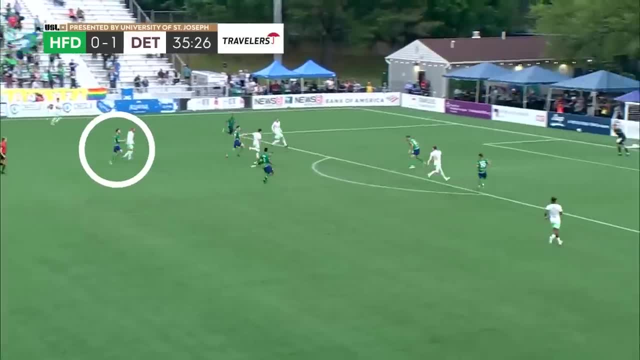 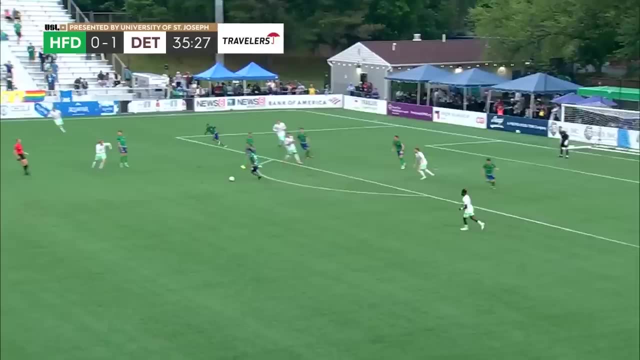 get a goal, which is great, Fantastic Save. next play here. Great tackle from Kaveh uh immediately into JP. I'm just checking over my shoulder because I'm guessing that I'm about to get this ball As soon as this player starts to leave. I do get that ball. I'm able to turn because I've 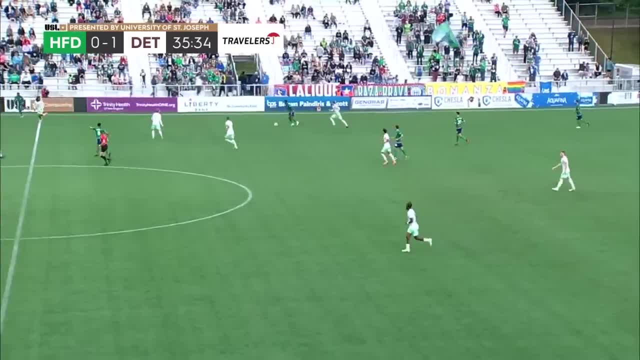 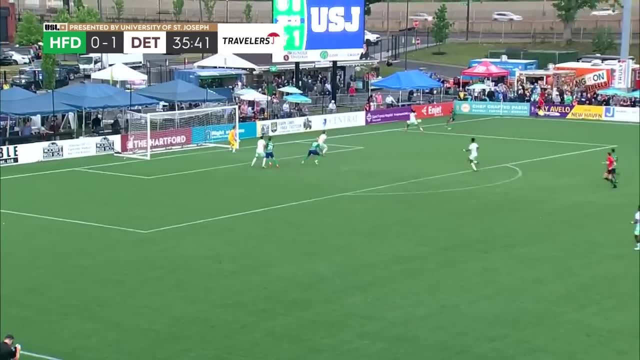 checked my shoulder. I played immediately out to Prince Sadie, our right winger, And I just stay in the middle to uh to support that. And that's a great ball through into Rideau And right here a B three chance to uh to score here and a great, great defensive effort, I think, Antoine. 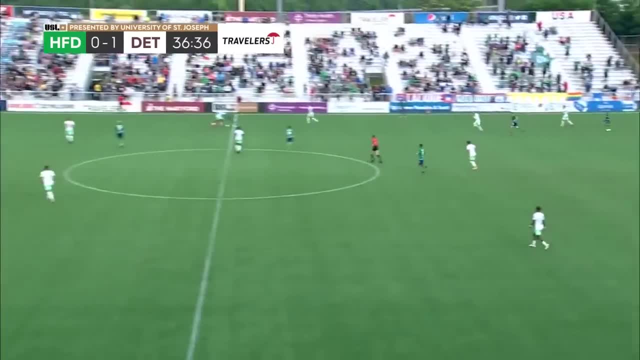 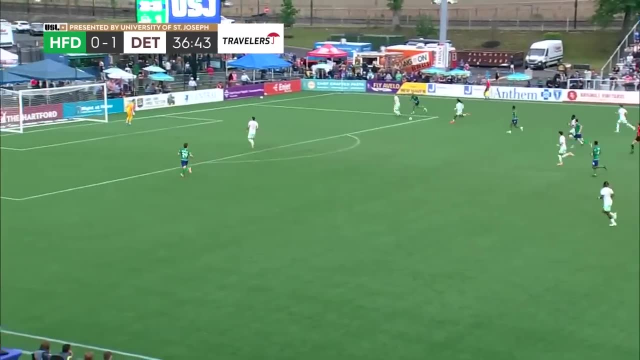 comes in fouls, The keeper ends up being uh Detroit city's kick there. but good play, Great play, Uh. and then header into uh Kyle from Prince Kyle takes him on one V one in the wing. It's a great ball into Elvis. Great defense there, to be honest. And then it bounces right to Antoine. 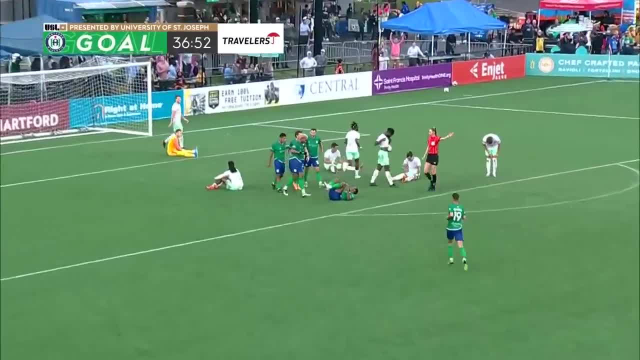 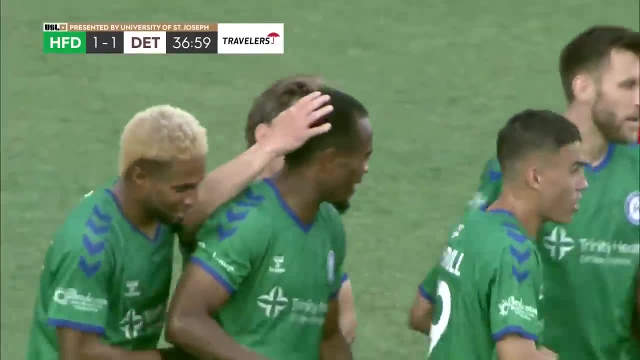 Hopeno who scores on his old club. So that's a great from Antoine, Great finish, You can see two even on the finish. like he opens up, Everybody's expecting is: you're going to go far post and just cuts that across his body, goes to: 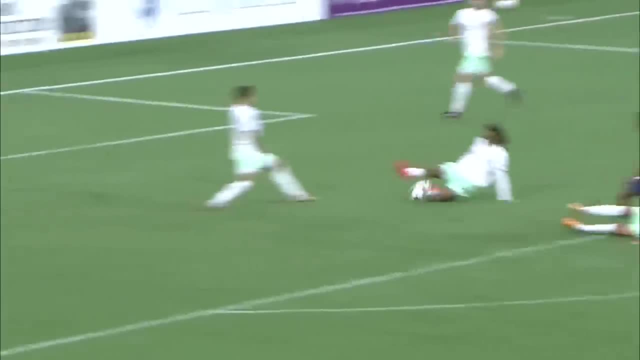 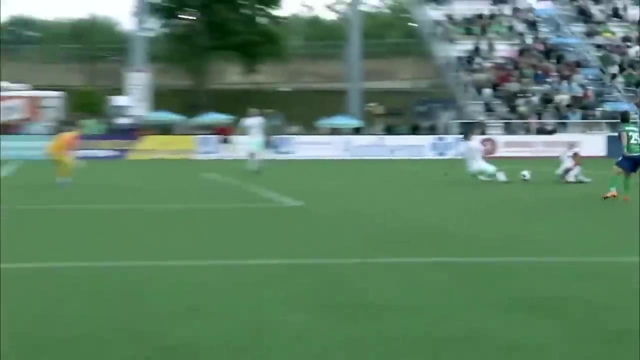 the near post. really good finish here. You can see again here. it is Great tackle, Good block, Honestly a little unlucky- from Detroit comes right down to Antoine right out of the six yard box- And you can see what I'm saying. He kind of like opens up his body and then just goes near. 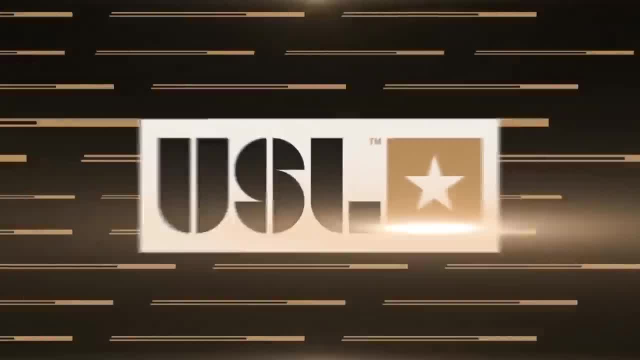 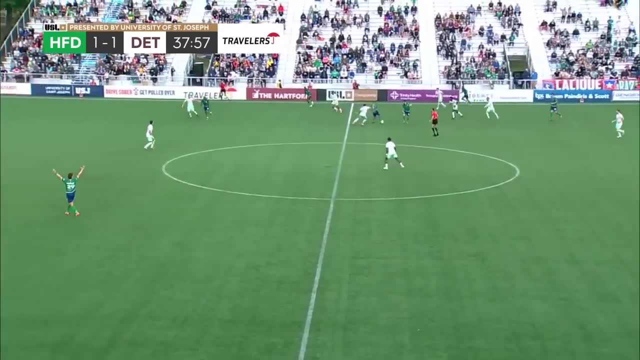 post with that shot and, uh, fools the keeper- Great goal. So now we're tied up, one one and honestly kind of had a rough start, but we respond. well, now ball pops to me kind of tackle with the outside of his right foot, I continue my run inside And now we have three V two Now here. 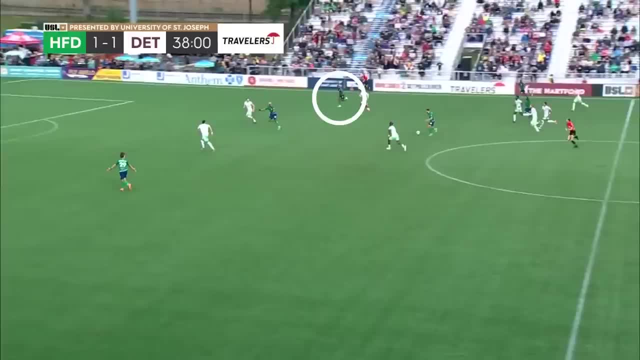 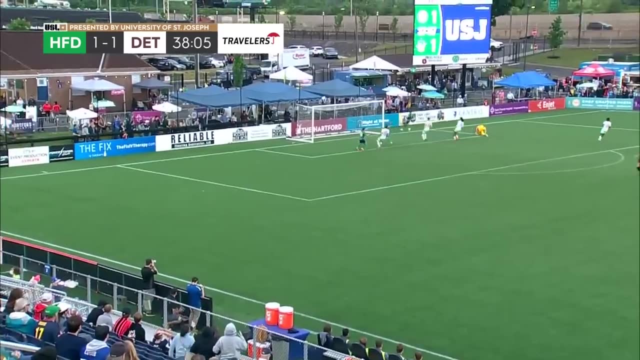 Antoine really is calling for the ball. I see Prince going in behind. I think Kyle's marked here, So I'm gonna take one more touch and then try to thread it through to Prince Sadie, our right winger, And I think that's a good ball. I just think it's a little bit over hit, It's, it's. 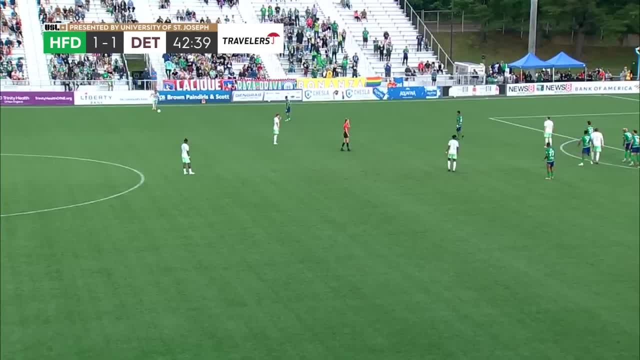 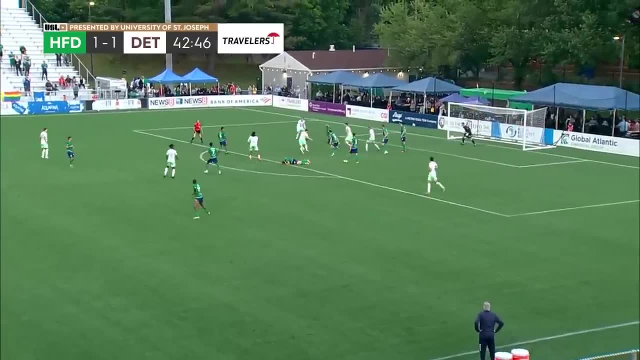 you know I put a little bit too much behind it, but still I think that's a good idea. I don't think that's, uh, the wrong decision at all. Now ball pops out into Antoine top of the box and he: 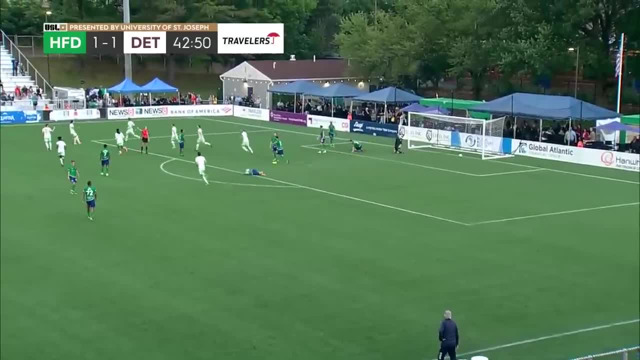 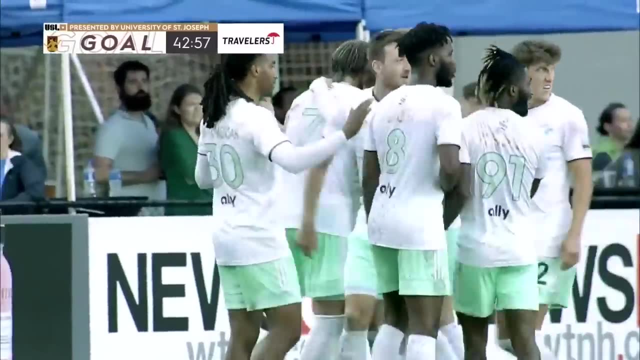 kind of gets elbowed here. Kyle fails to clear it there And unfortunately it gets unlucky, gets stuck under his foot and then Detroit capitalize here. Now I hate to be the guy that complains about calls from referee. I I think it's so lame, but I really do think this. 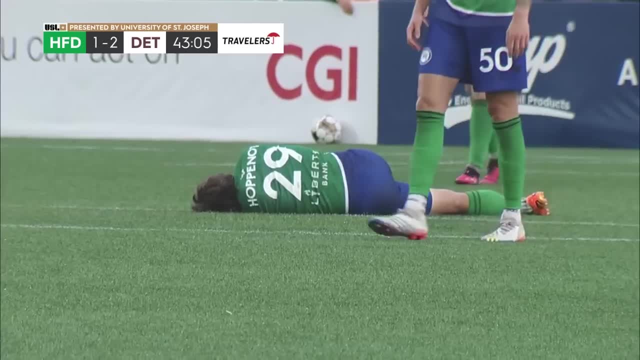 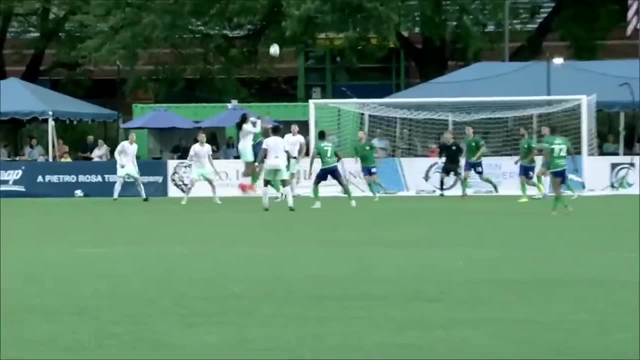 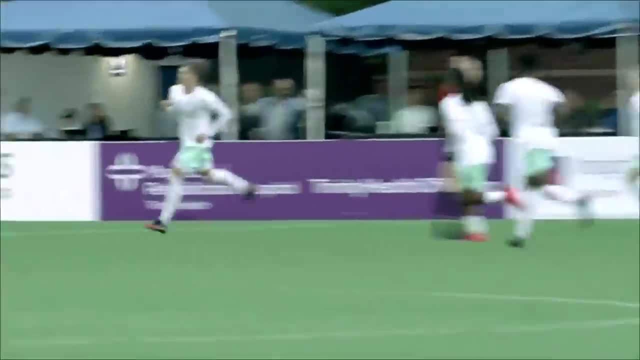 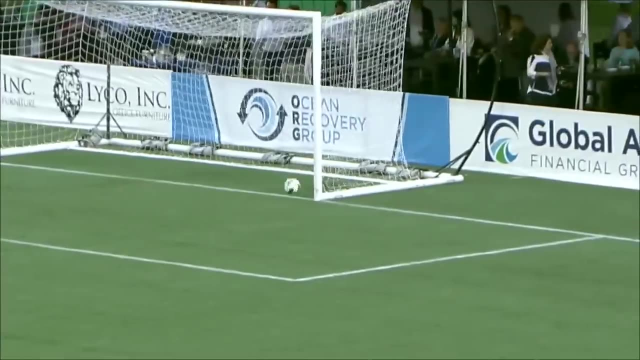 I said I hate. I'm obviously so biased being a player for Hartford. He's going down a goal here, but I think that's a pretty clear elbow and foul top of the box. Um, but you know I hate, you know. 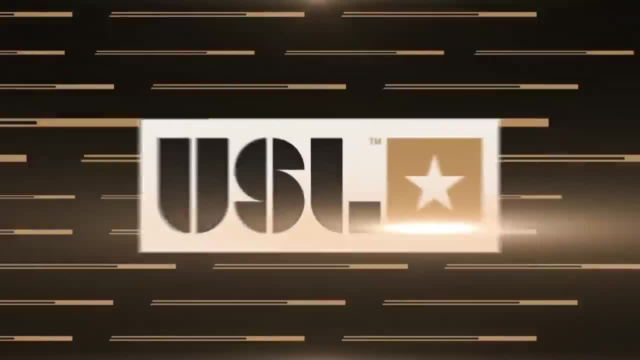 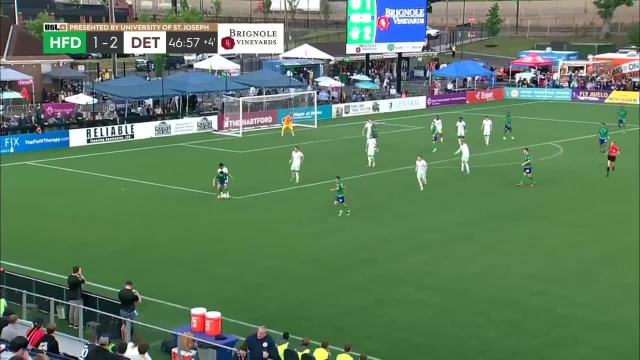 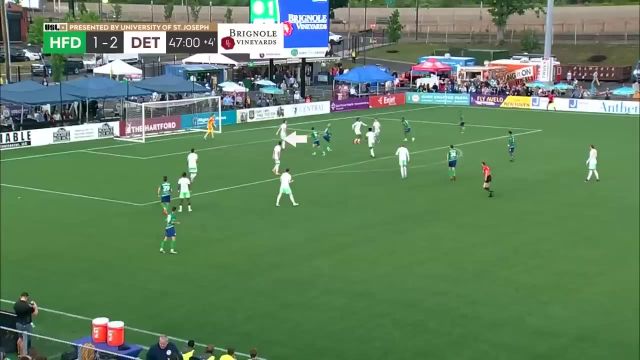 I don't want to take anything from Detroit. It's a good win there. Ball falls right to uh Simonson, and then he's able to uh to put that away. Ball pops out to Antoine. now Great ball into the back post here. Now I always kind of make the opposite movement and it's going over my head. 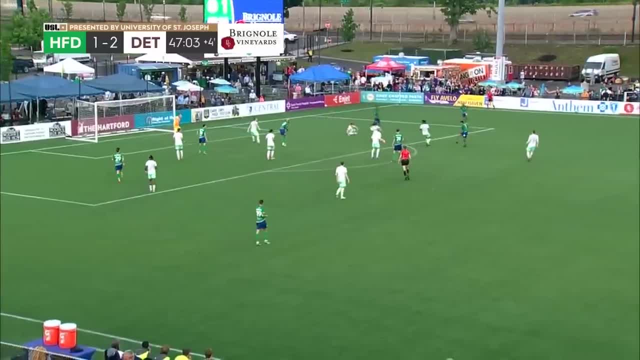 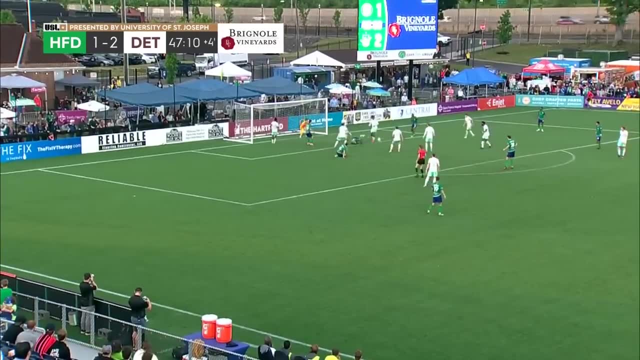 recycling my run- I'm sure you guys have heard that- recycling my run into the the center of the field. So if this happens, another great cross in. I can just win that header. And then Kyle almost wins that, almost gets a shot on goal there. So that's always my cue If the ball goes above my. 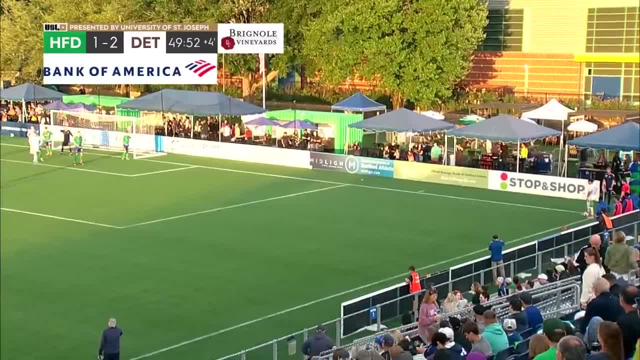 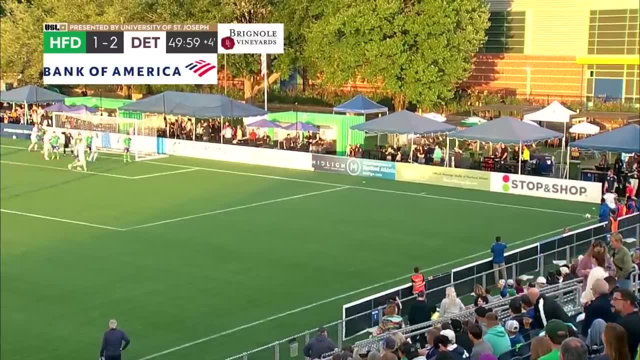 head. I'm cycling in trying to get that second ball If it is headed back into the six or across the six yard box. Now, 50th minute, still in the first half, um stoppage time. Maxi Rodriguez with. 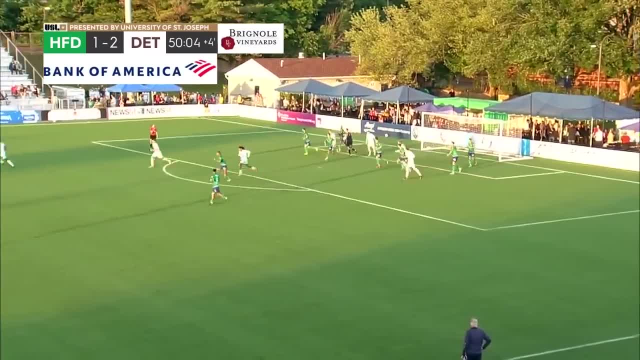 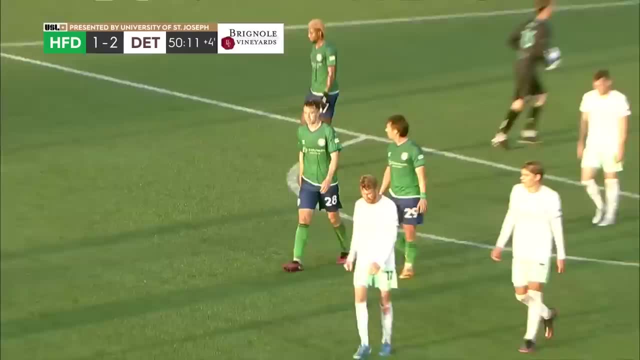 a corner, kick right into the box, Joe Rice collects it And then that is the end of the first half. So, uh, not the best half from us, Um, but Joe Rice with a big penalty save. it could have been worse. I think we could have capitalized in a. 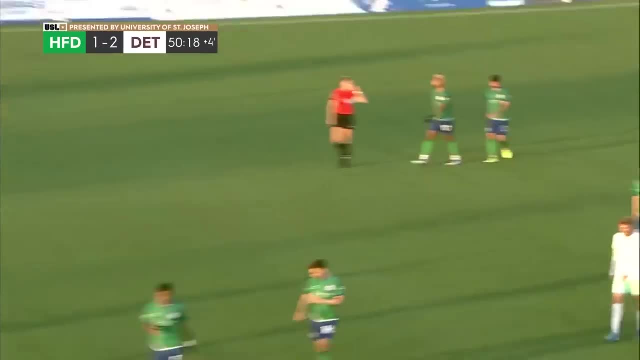 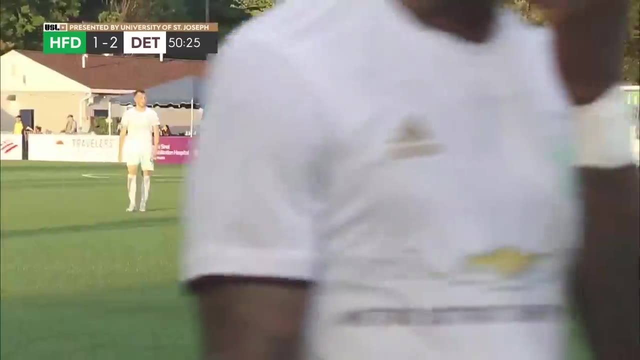 couple, uh, key moments. and then you know, obviously I'm biased, but I think that was a foul on Antoine with the the elbow. He personally I think it was a good half. I think there's again a few times where I'm just feeling a little unnatural and not used to having pressure and 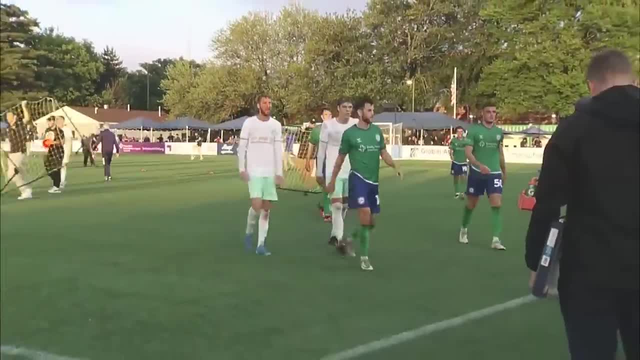 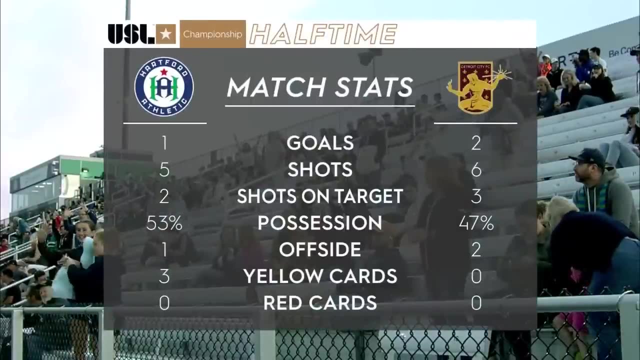 three players surrounding me at times. If I can release that ball a little bit quicker, I think it'd be a great half from me here. The match stats from the first half: um, pretty even. I mean five to six on shots, two to three on shots on target. possessions, pretty much split. So it's a 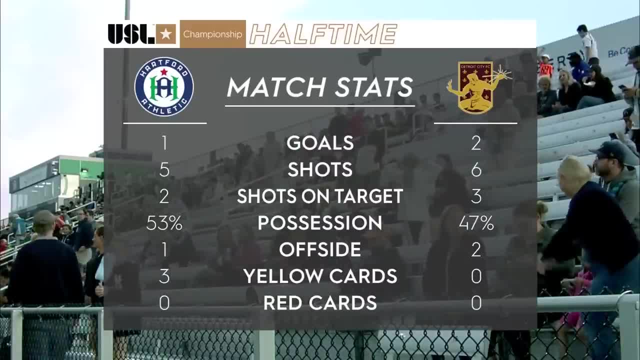 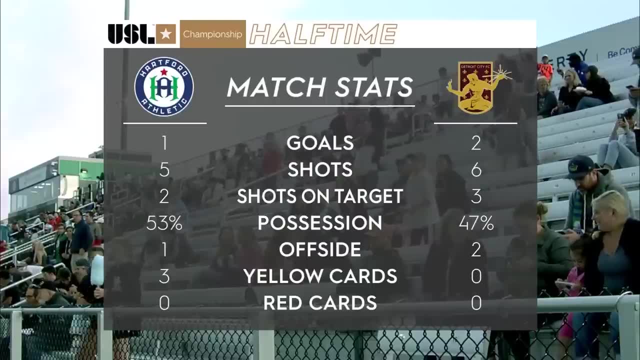 it's a good game. Um, Detroit just capitalized on their opportunities and we've only capitalized one of our opportunities. but it's a good half And hopefully we can go into the second half a little bit stronger. Oh, and actually I got to talk about this too In the second half. 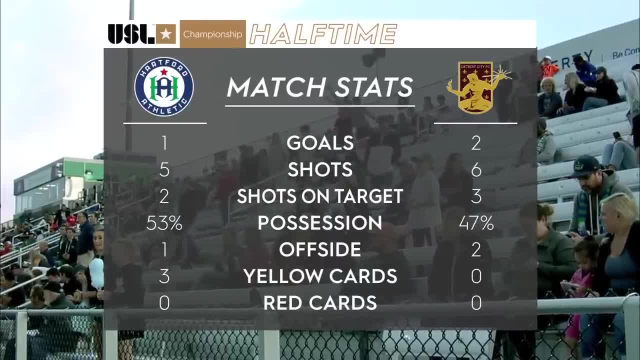 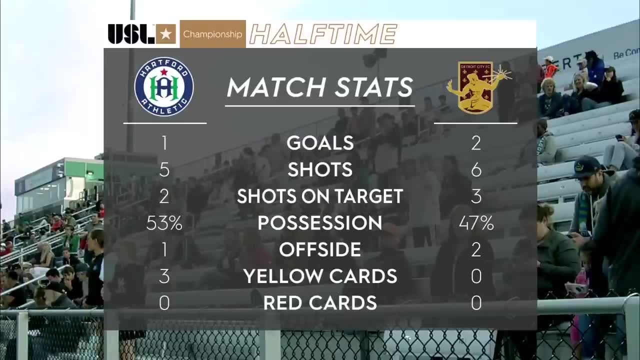 we make a few substitutions and I get pushed back to right back. We go four in the back. Now I'm playing right back- my natural position. So I'm pretty excited to to get back there. And that's not to say like I didn't like playing center mid, I really enjoyed. 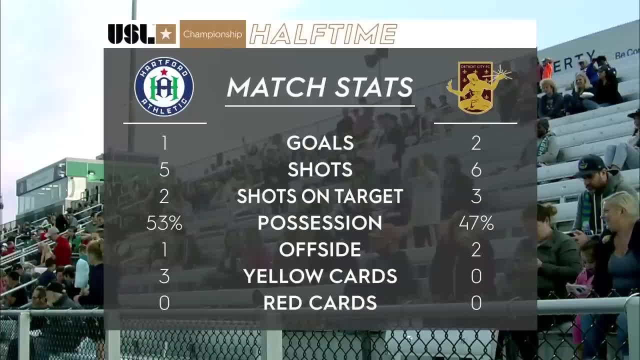 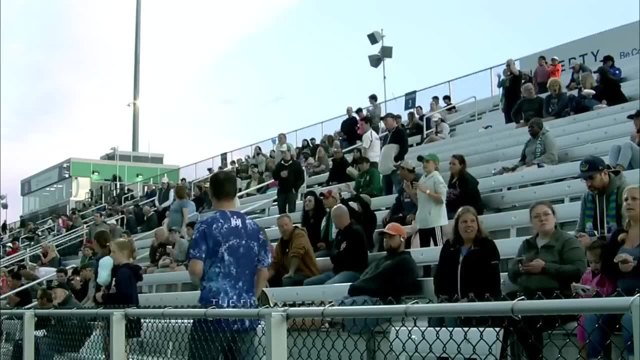 that getting involved in the attack, trying something new. It's a new challenge. Um, wherever the coaches want to put me, wherever they see me helping out the team, I'm happy to to try out. Um, but yeah, definitely I think personally I enjoy playing right back the the most, So here. 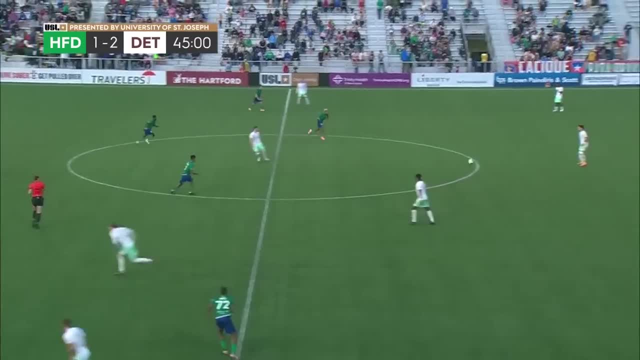 is the start of the second half. Detroit city FC. It's going to start with a kick. They're gonna play it back to their center mid Maxi Rodriguez, who does a great through ball, And, uh, we do not defend this Well. 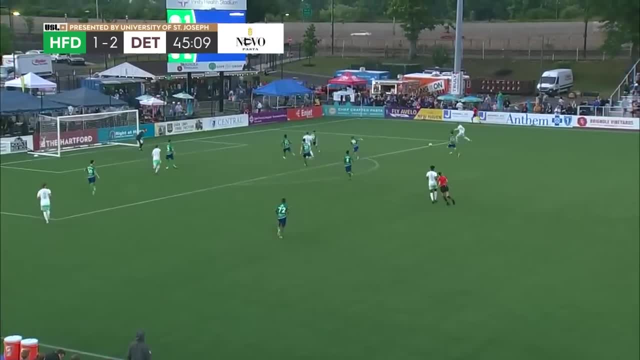 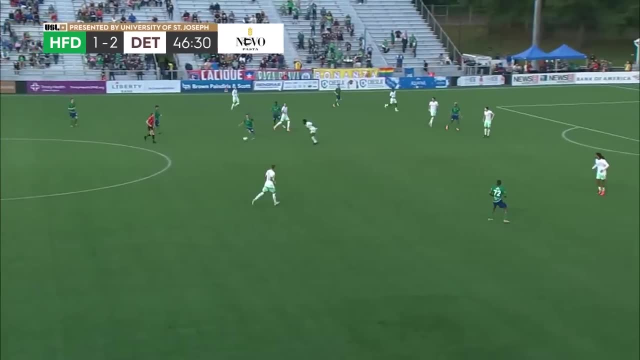 get countered, attacked. We tuck in defensively, The ball goes wide, great ball in, and then they almost score off of it. So that's a terrible start from us. 15 seconds in, we almost concede a- uh, a shot on goal. Here's my first touch in the second half: receiving the ball from my, my left. 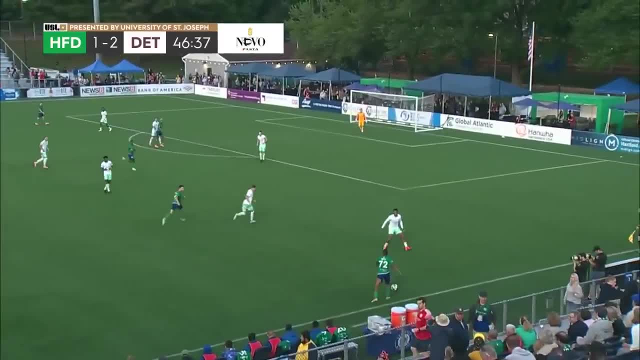 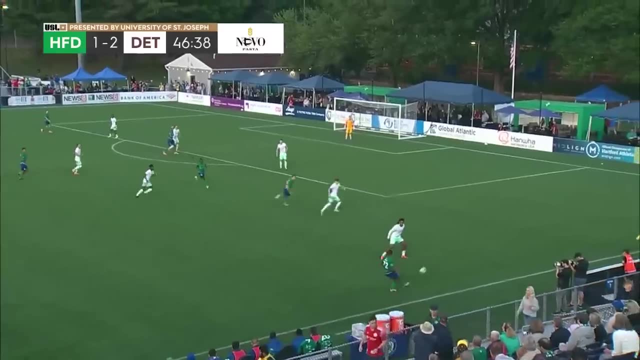 back, actually passing that out to my right winger, And as this right back comes in this center, back, say centrally, there's this big pocket of space here, So I'm going to take that space running behind. This is like a uh uh under lapping run. It was a great ball from Rito. I'd check over my. 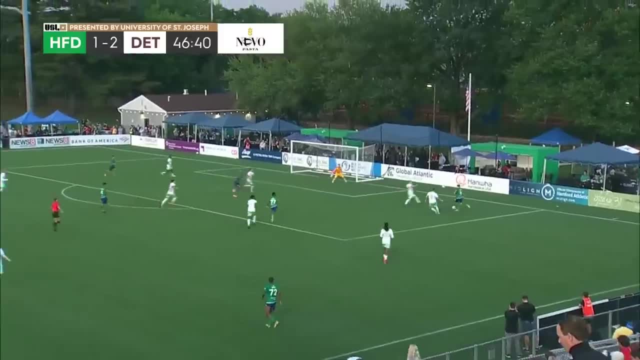 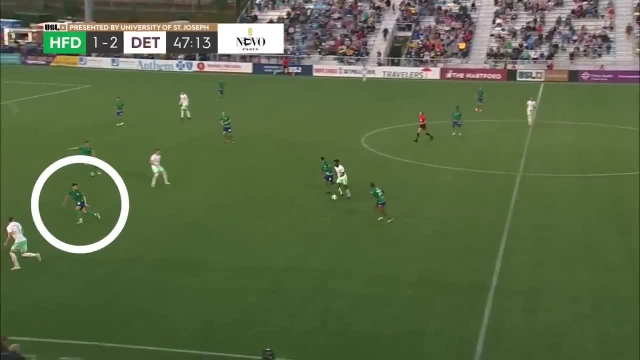 shoulder just to see where my runners are. I noticed I have another center back coming very hard. So just one touch that on the ground and dangerous area. I think that's a great spot to score And unfortunately JP just doesn't put that away. but it's a good effort from him. 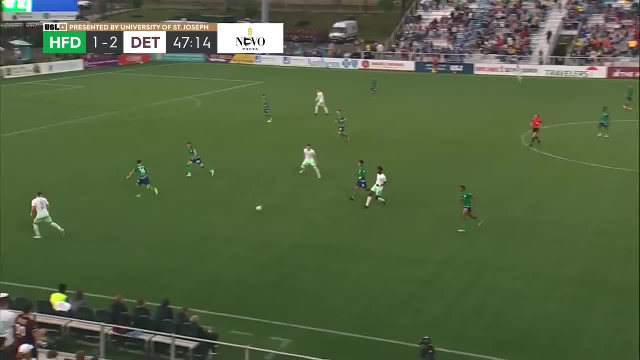 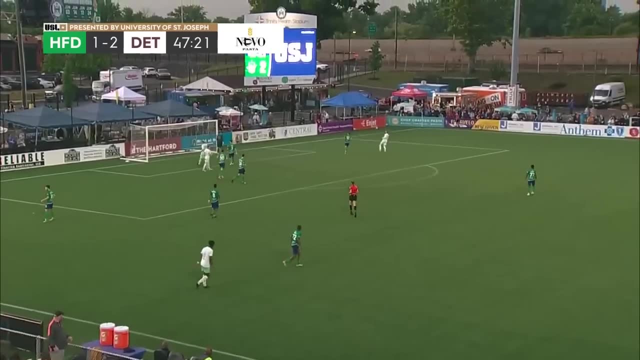 And then here my- uh, my winger is making a run in behind, So I'm just going to tuck back, drop back and then just stand them up for some wide stand them up. So great ball in, but you. 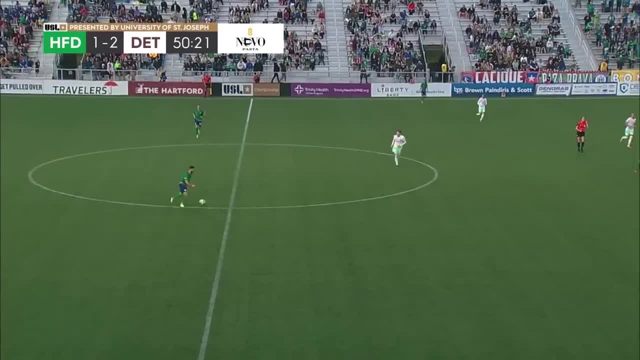 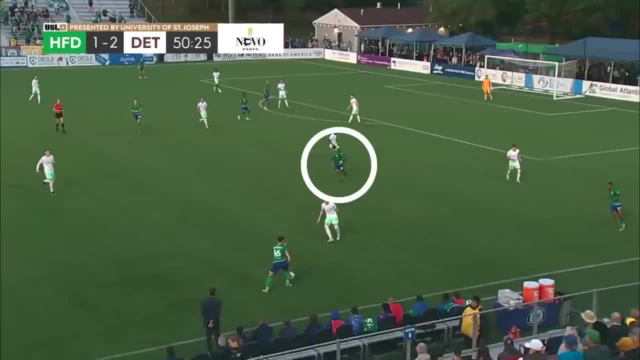 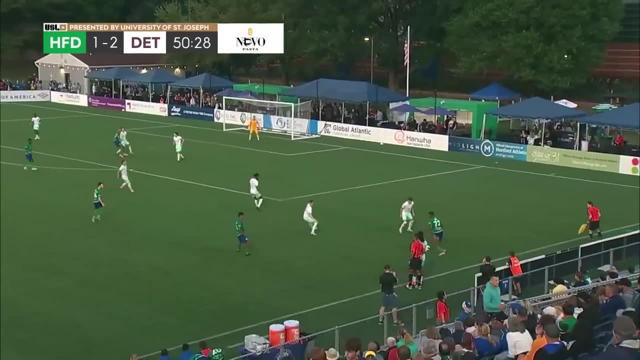 areas receiving the ball Now opening up. looking wide, I have JP coming towards the center, but I also have a Rito right in this pocket, right here too. So I'm playing to Rito and I was about to make the under lapping run, but I didn't think the space was there now because they kind of 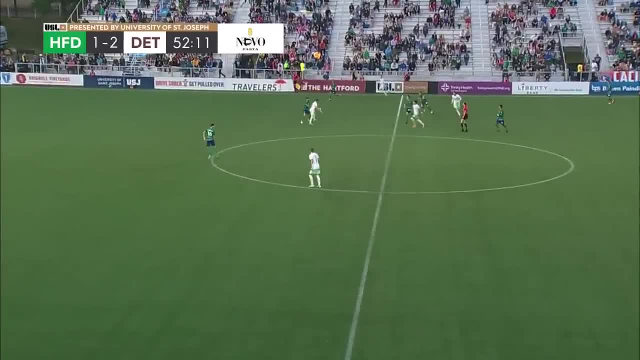 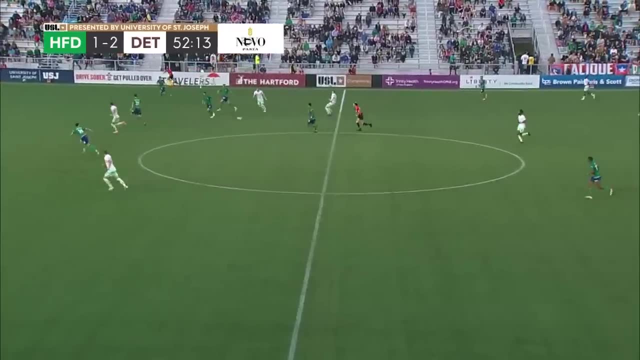 probably, uh, changed from the first time. I did that under lapping run, So I kind of just hold back now. now, here, center back goes to the ball. I'm just tucking in behind for a little bit of support in case this happens, And then I'm going to tuck back, drop back, and then I'm going to 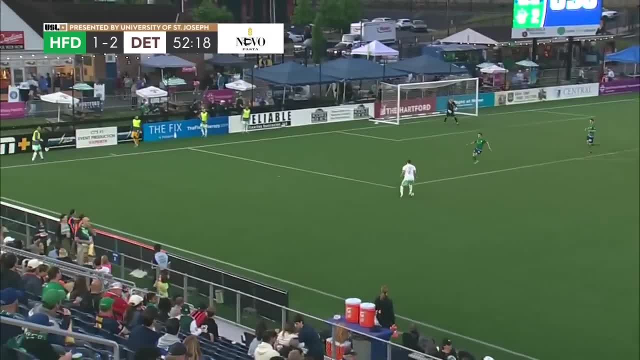 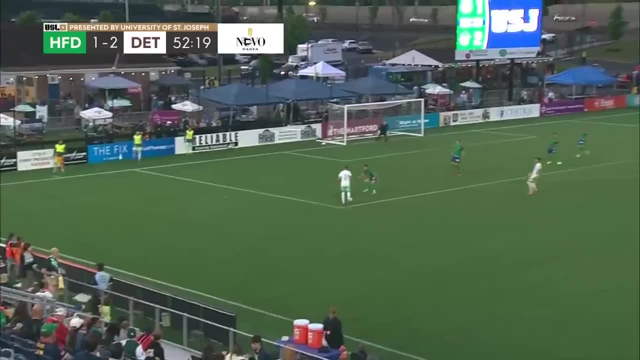 this is exactly what happens. Ball comes into max, He plays it wide And then once again just standing up, this winger one V one, forcing them wide, cutting off the inside a little bit and just waiting to see what happens here. I don't want to lunge in, just blocking any potential shot. 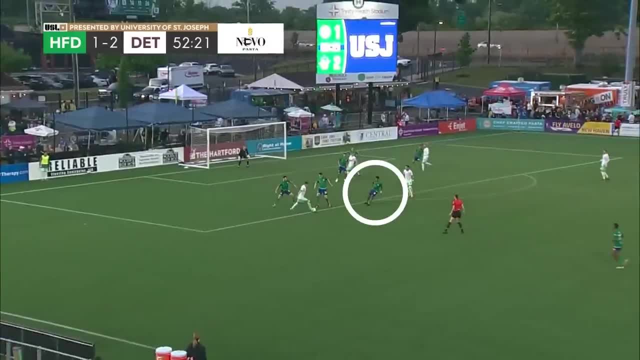 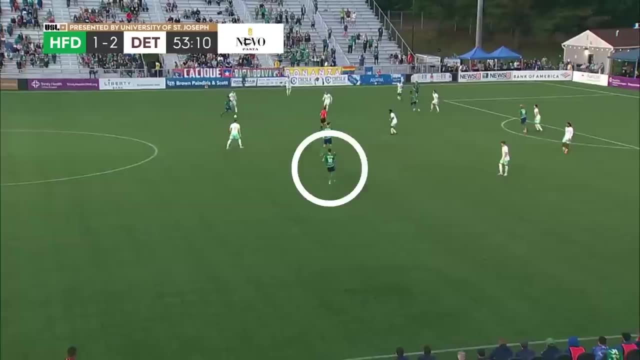 Connor does a good job to come over and make this a two V one. even G JP comes over to make this a three V one. And this is a really good team defense forcing that ball back. And then Rito comes in and wins that ball and drives forward for the counter attack, So that's a really good. 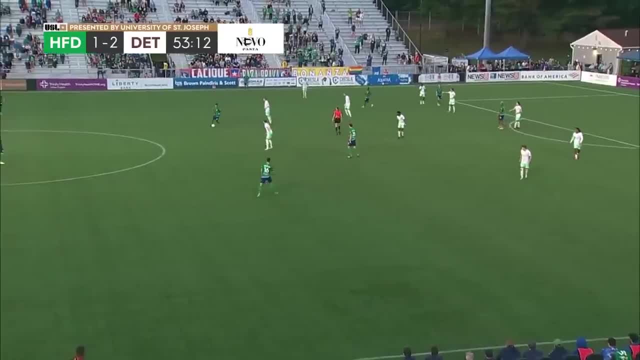 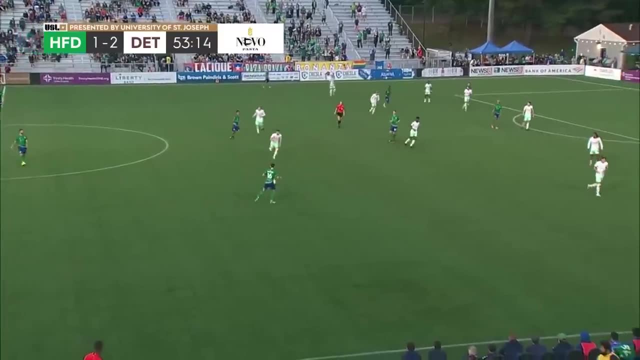 team defense. Just checking over my shoulder. Now more inside here, Cause my winger, Rito, is high and wide, So I don't want to be on the same plane as him, So I'm gonna be inside Now I can take my touch forward, because I want to get in front of 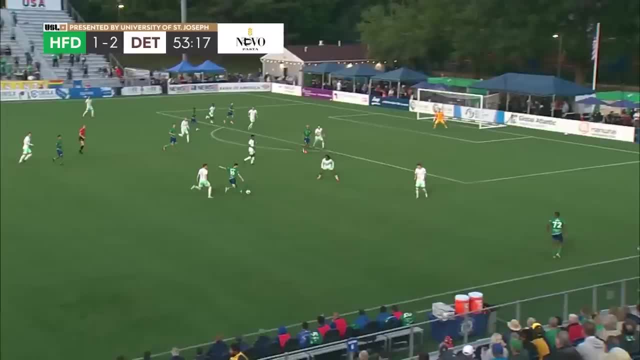 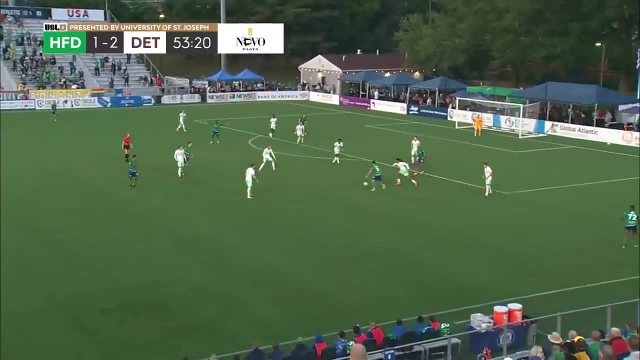 this guy here, drive forward And I'm just going to cut the ball right here into Connor, Who's in a good spot top of the box. So I'm going to chop this ball right into Connor and he's going to play me right back, take my touch inside And then I just quickly see Antoine, here He's in, I think. 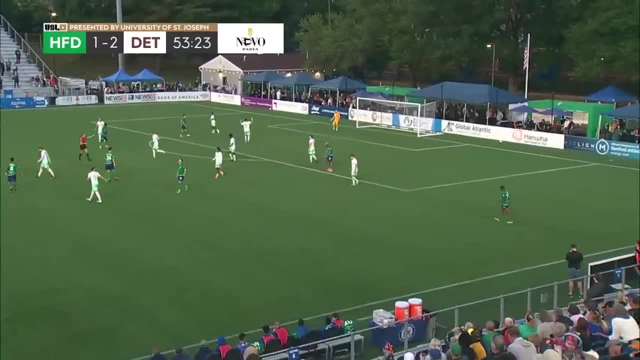 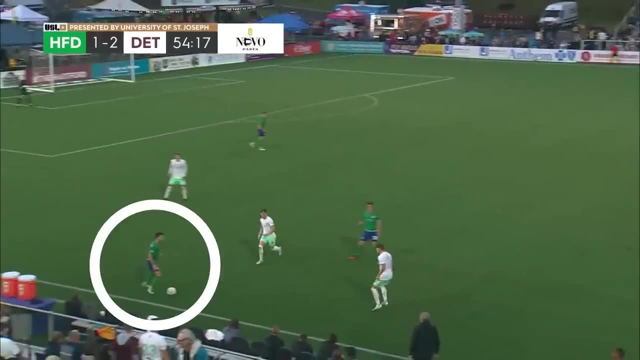 he's in an offside position and that's not a good ball. It's a little way too deep on the long page. but I just thought I'd try a little hook, a little chip, a little clip into the, the back post here, saving this ball from my center mid opening up. Now I have a lot of. 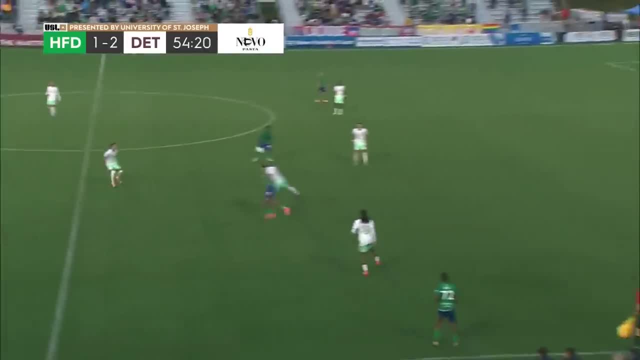 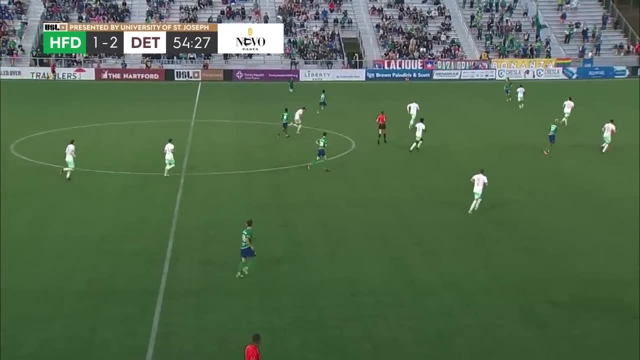 pressure here and I just am going to kind of curl this ball into that pocket of space. And Kyle Edwards, my striker, does a really good job to win that ball And we get to keep the ball. now attack up this left side. Stein washer with the- uh, with the drop kick, comes all the way back. 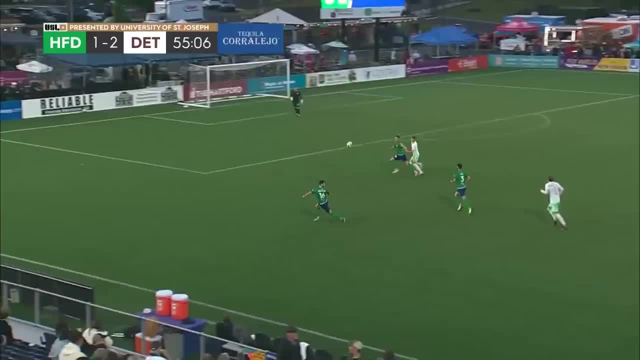 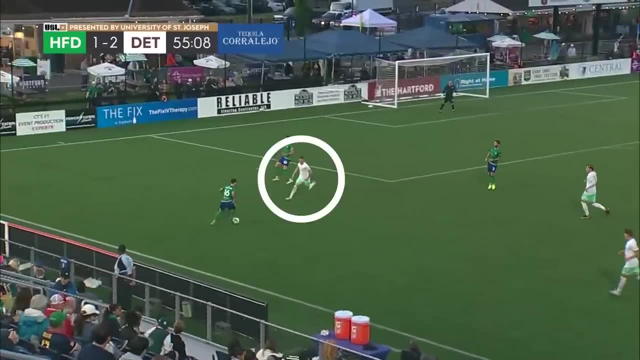 I'm telling Nile now is like screaming: He's got it. So I'm checking my shoulder Cause that header is going to come to me. I want to turn open up and then just take my first touch in front of this striker, in front of him, So now I can just put my body in between him. So if he wants to win the 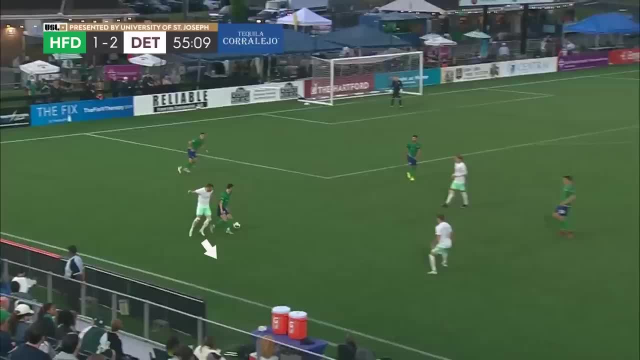 ball. he either has to go around me or through me. He opts to go around me And as he goes around me I'm going to turn away from that pressure inside, And so I can go and keep the ball and play it back. 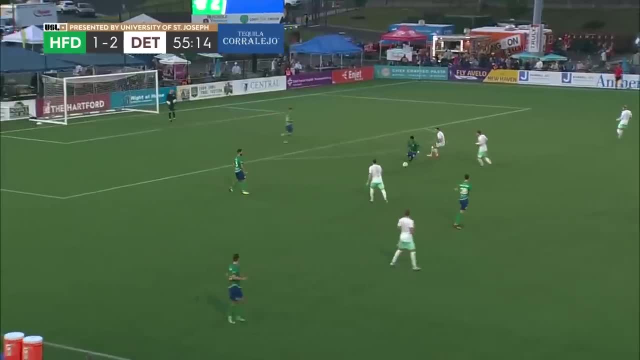 to Nile now. So it was a very simple play, but just keeping the ball in those situations is is really important as a as a fullback And as a defender. you don't want to just clear those balls out all the time. 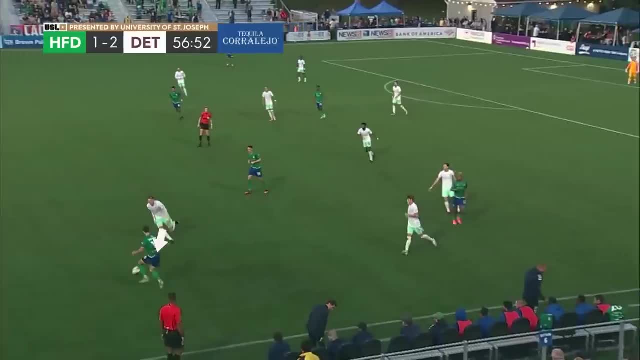 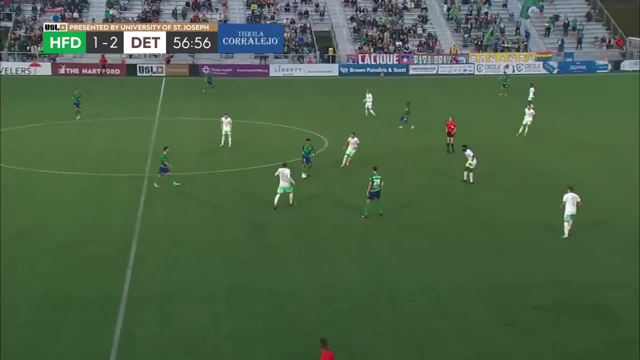 Uh, the ball comes right back into me. from Kyle's a great ball. You can see a lot of pressure. So again I'm going to take my touch, kind of against his momentum, away from him. And as soon as you take that first touch, usually strikers, wingers, they, they kind of give up. So if you can get, 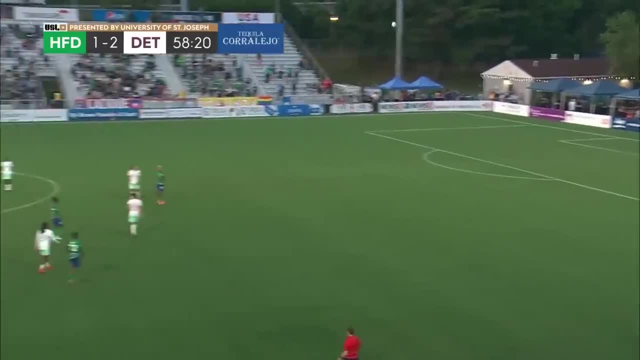 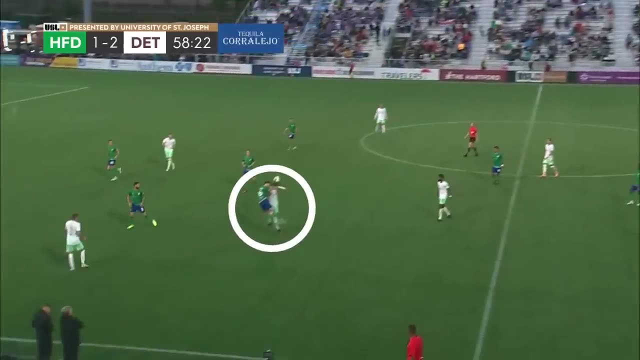 past their initial pressure. you usually can get into a spot then where you can kind of then make a much easier pass, trying to win this header over Simonson. Um, he flicks it on here and this is a great run from Reese Williams, great touch from Reese Williams and then a great pass. 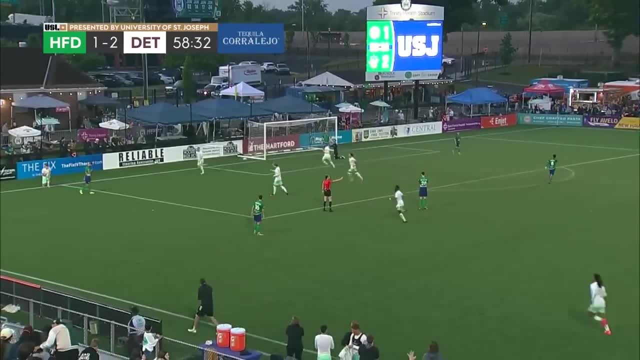 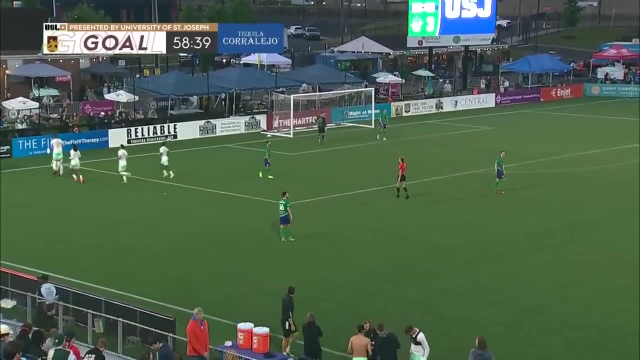 Uh, and then he just beats, uh, beats us defensively right exactly into the uh, the one striker in the box, And then they go up three, one on us, 59th minute. So it's, it's- I mean, it's- frustrating. 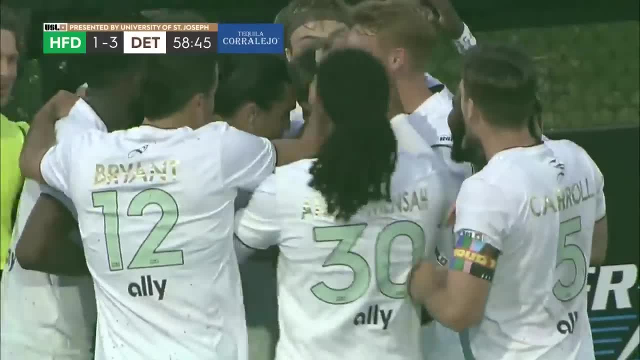 It's not been, it hasn't been great. Um, and plays like that. I mean it feels like we're doing well, we're starting off the second half well, and then they have one play, flick on, and then it's just a. 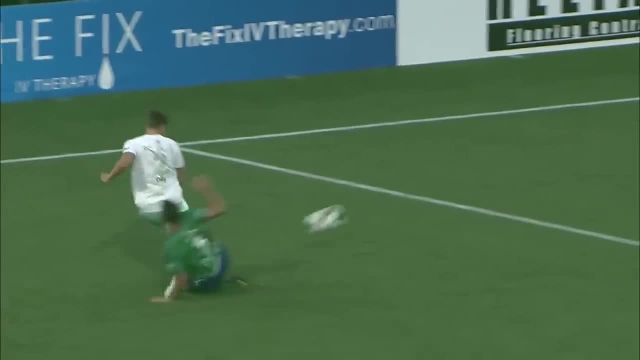 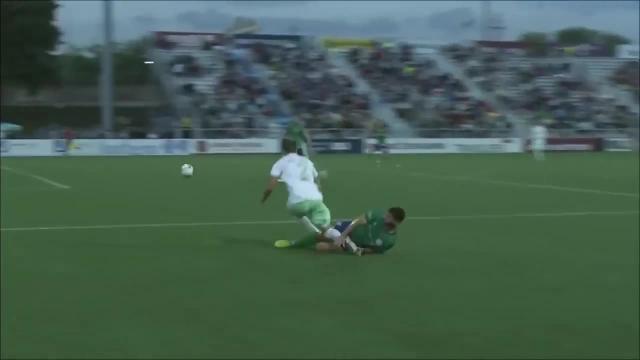 great counter attacking sequence, And again I mean Reese Williams, the touch there, the cross there and the finish. It's all. Yeah, Yeah, Yeah, Yeah, very, that's very good, That's a great ball in. Um, yeah, I mean, the goalkeeper doesn't have much. 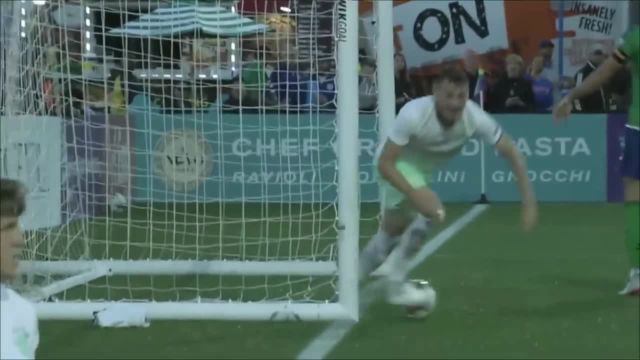 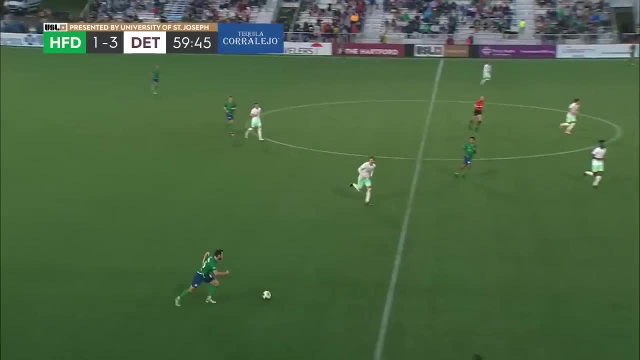 of a chance there when he when the shots coming right on top of your six yard box. Um, but anyway, moving on, here's my next touch in the game. Just calling for this is pretty much right after the kickoff, receiving that ball. Now I have tons of time, tons of space. I'm going to drive forward. 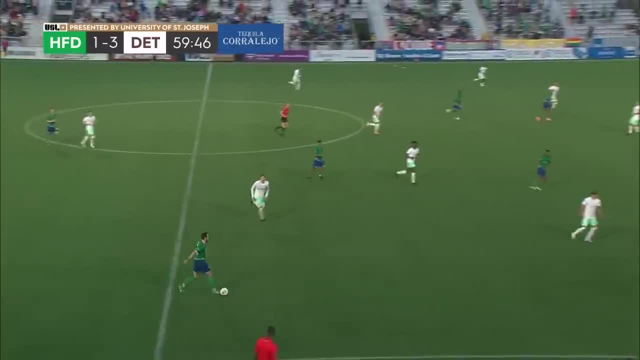 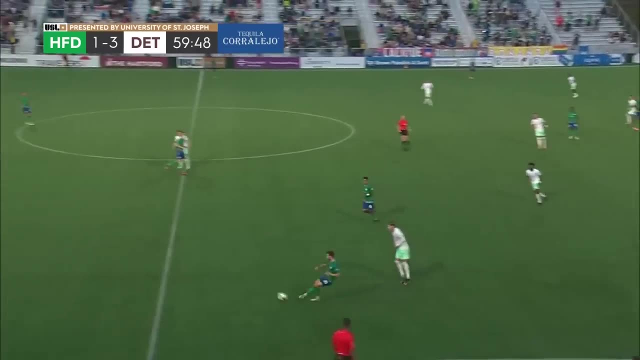 into this space just to move my team up a little bit up the field. driving in And, as you can see, one, two, three, four Detroit FCs- uh, players, right here it's closing down. So instead of running to that pressure and trapping myself before I get there, just cutting the ball back. 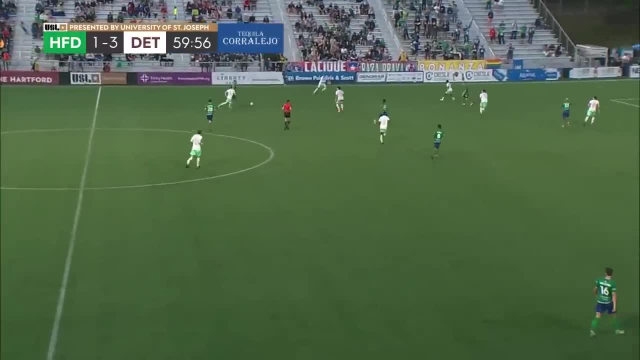 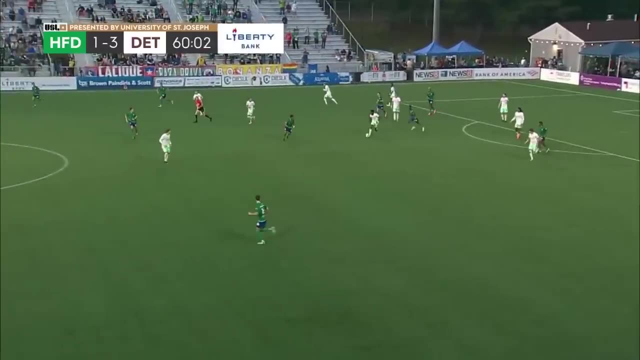 playing back into my center backs, being patient, So we can circulate the ball and try to find um gaps and holes up the- uh, the left side, just like this. Unfortunately, we don't connect there And then here as we lose the ball. instead of running towards the ball, I need to tuck in. 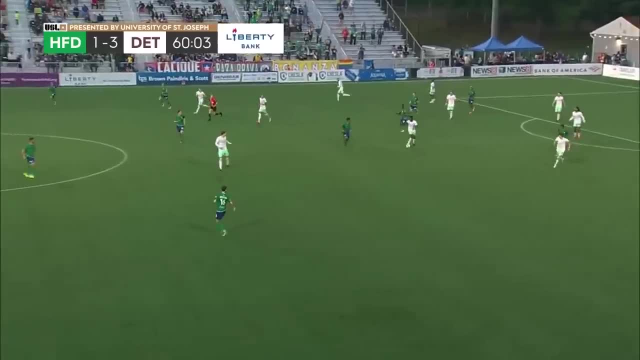 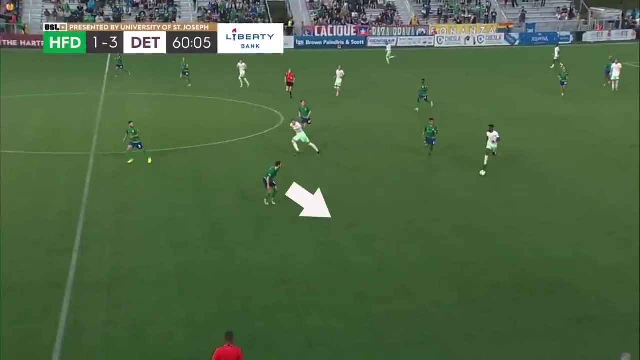 tuck in centrally and force everything out wide. That's. you know, it's pretty much what most teams do: tucking inside And forcing this play wise. So you can see my positioning. I tuck inside. Now my body position is forcing him this way, JP is forcing him this way. We're just getting ready to kind of put him. 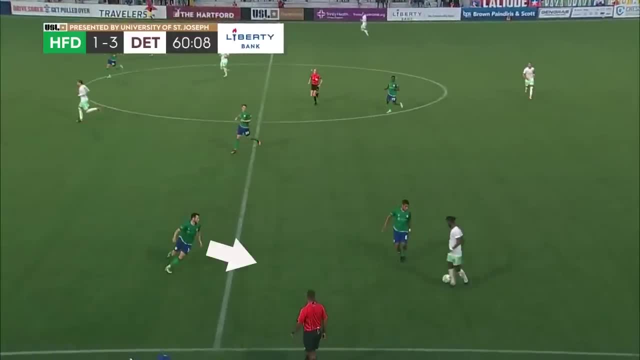 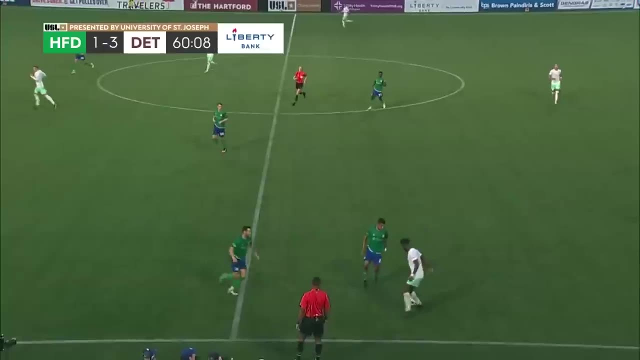 to the line And as he keeps on getting closer and closer, this is now kind of a cue for me to fly in here and make this a two V one and try to win this ball. And Connor's in a great space right here, just in this pocket, And he doesn't have much of an option- tries to play it through. 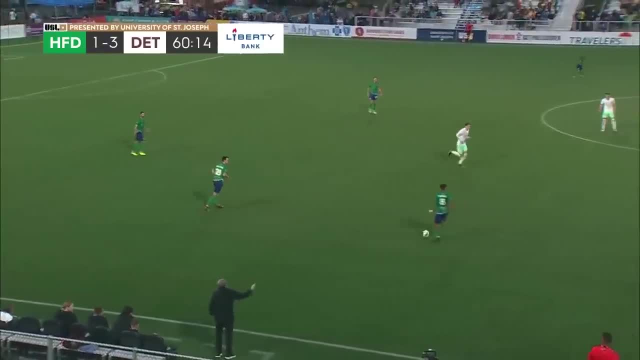 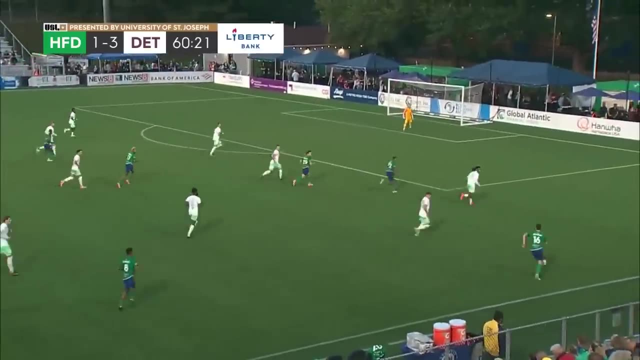 and Connor's able to win that. So I mean that's exactly why I cut the ball back just before. that is because you don't want to get in those situations where you get trapped like that. Now receiving the ball forward, taking my touch forward, looking forward, I just kind of am. 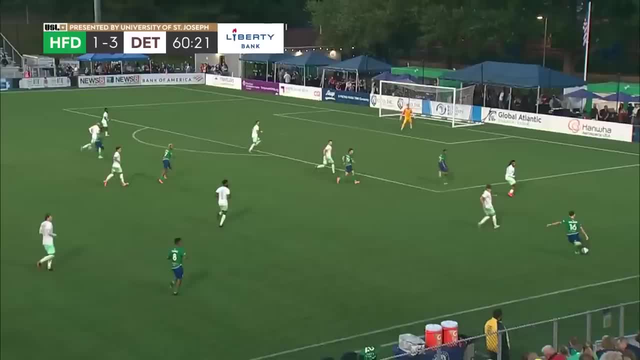 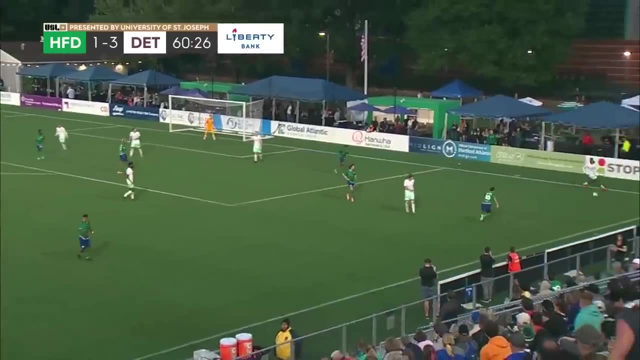 looking towards here, Kyle and Andre Lewis right here. It's not as on as I thought it was in the game. I don't think I saw this player right here, but I'm just trying to put it in behind Carol there, that defender who, who clears the ball just to put it in a dangerous spot and see if we 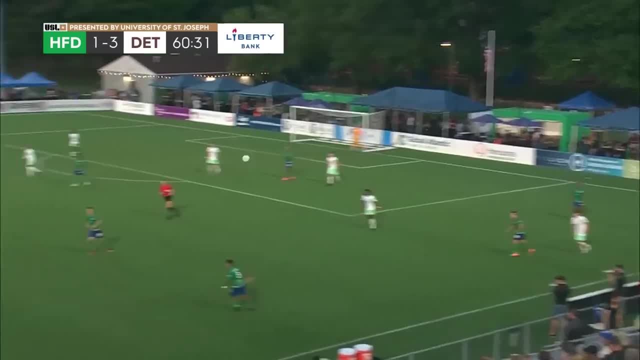 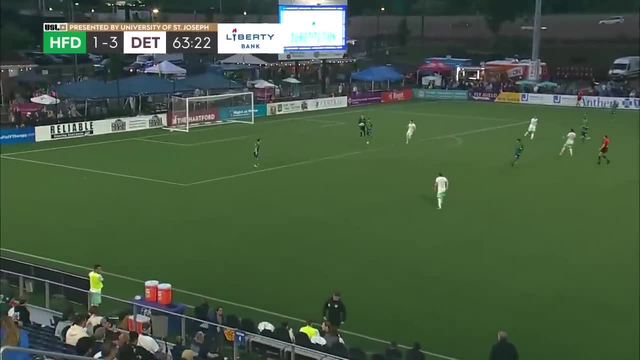 can get there. I don't think that really was on. I think I could have made a better decision there, but probably was getting a little impatient, especially being down three one and trying to create something which you know. you gotta be patient If it's not on. I gotta be smarter with. 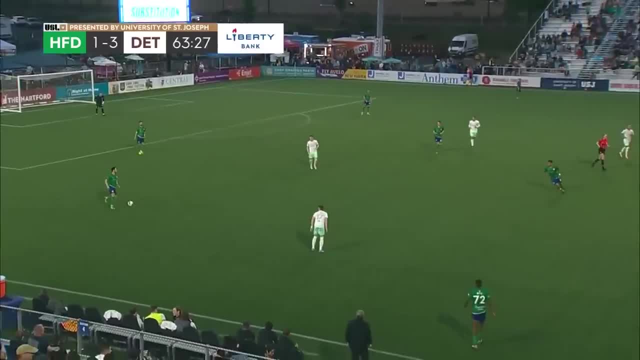 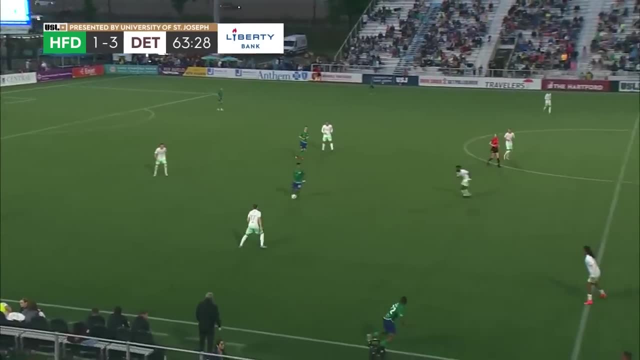 that decision, receiving the ball, tons of time and space looking forward. Now, here you can see this player is kind of cutting off the line and taking this, this space, away, Cause we've played down the line a few times, So I'm just going to play in the middle, whatever they give you. 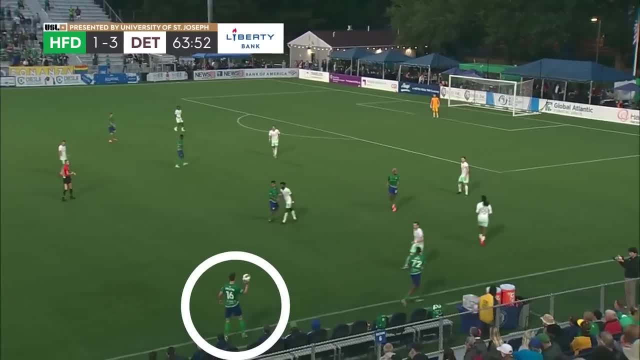 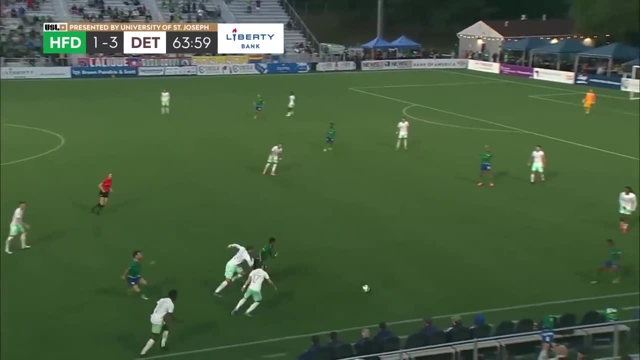 you kind of just go in the opposite direction. Unfortunately, ball goes out of bounds. I think this is a few seconds later the ball comes back to us, just winning that tackle, winning the second tackle, and then just get a little bit lucky there, Just kicking the ball into space for JP. 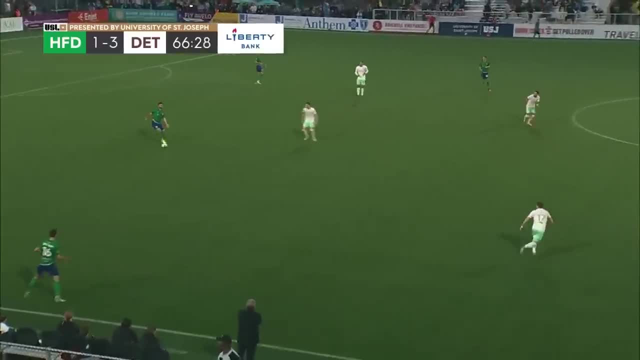 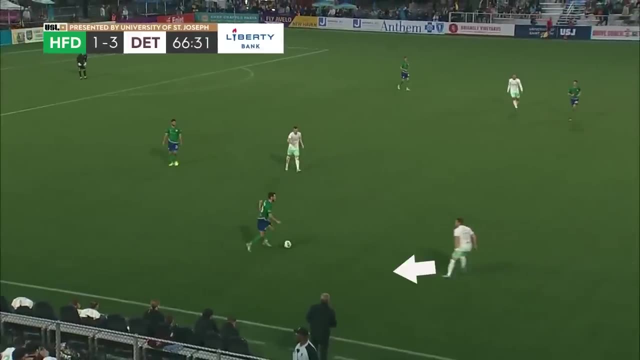 ends up being a free kick for us. right there in the corner, Receiving it from Kaveh. Once again, you could see this player rounding his run, cutting off the wing, and that's fine. If they round the run like that, it usually opens up this. 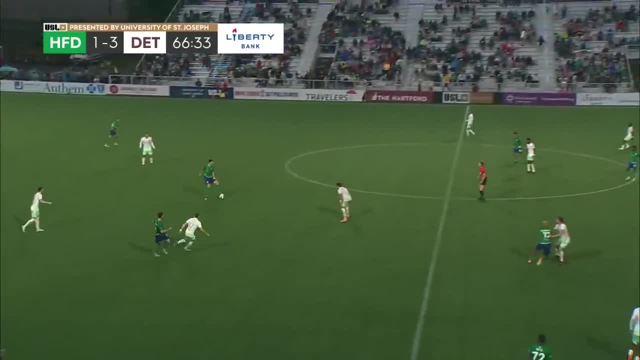 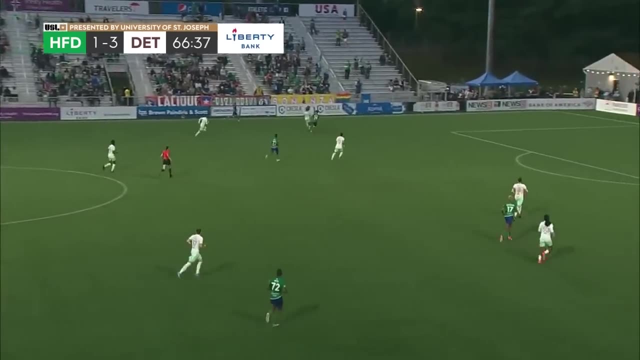 where you can drive inside and play in the center mid, And if they round the run the opposite way and force you to the line, that usually means you can. you can go down the line and try to find something towards your winger, or or, or, go that way. Whatever that, whatever the pressure is that. 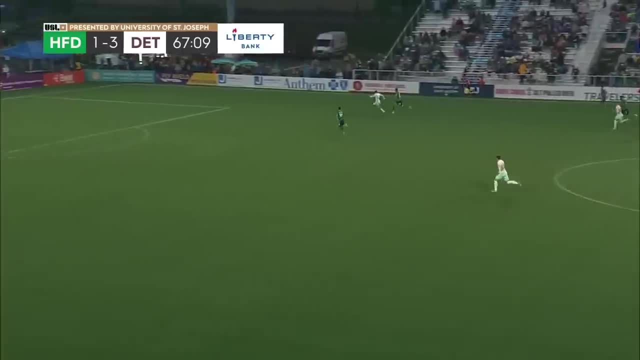 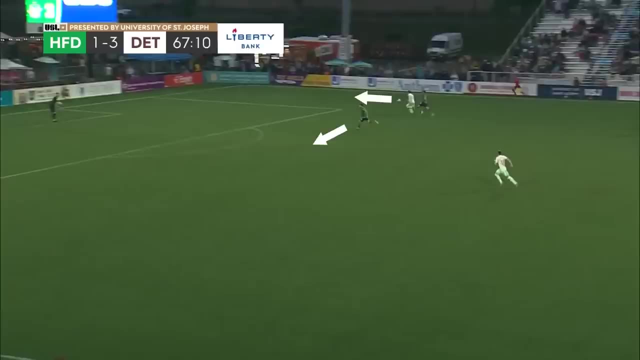 usually is opening up another opportunity. a little counter-attack here, And I'm checking my shoulder now to see where where there's room. So I'm going to go down the line and I'm going to see where the runner is. since he's taking his touch kind of more down the line, I want to stay. 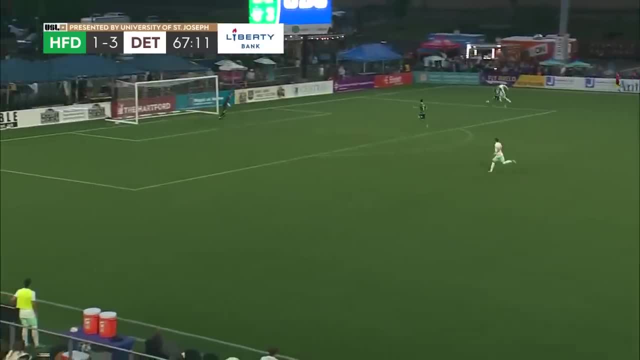 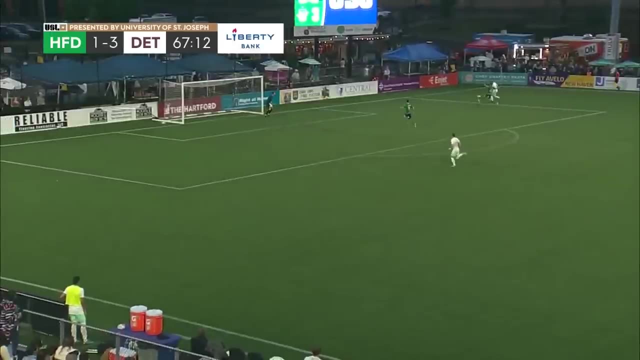 towards the center of the field, the middle of the field, because that's where the dangerous areas and probably where this ball, this cross, is going to be. So I put myself in a really good spot by noticing that run and not, you know, flying over there and trying to make it a 2v1. 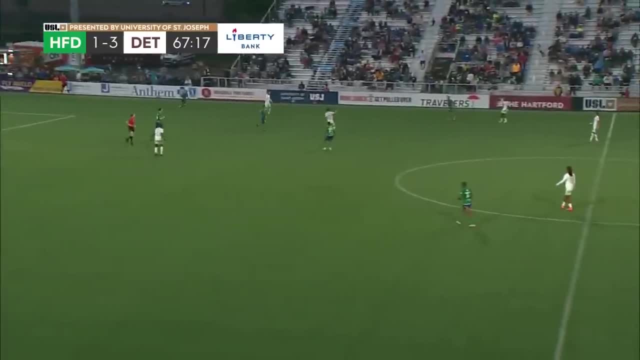 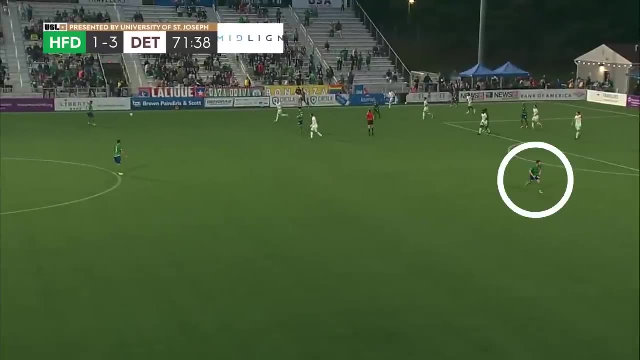 to just intercept that. And then I try to play into a. I think I was playing, trying to play JP, and just miss that, uh, with my left foot. but defensively the positioning I think is great. Now, here I was inside, I'm checking my shoulder, looking out towards my winger. 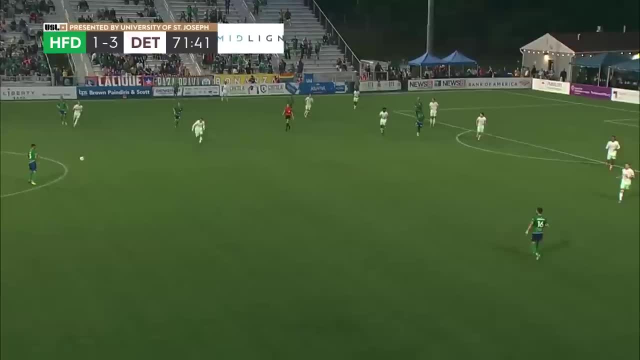 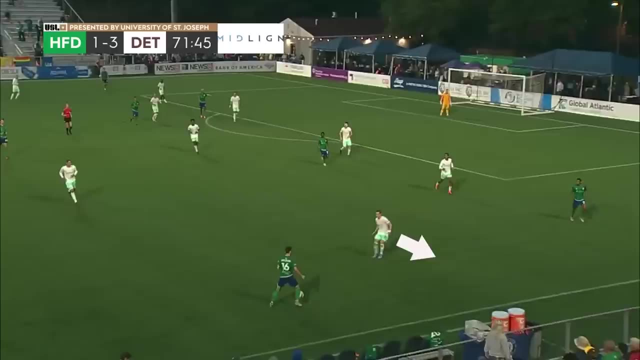 and coming out wide so I can receive this ball Once it goes into Kaveh. I can be in a good position now to receive this pass, As I received this once again. look at this player cutting off the wing towards Rideau So I can go opposite and cut inside now against that, just doing the. 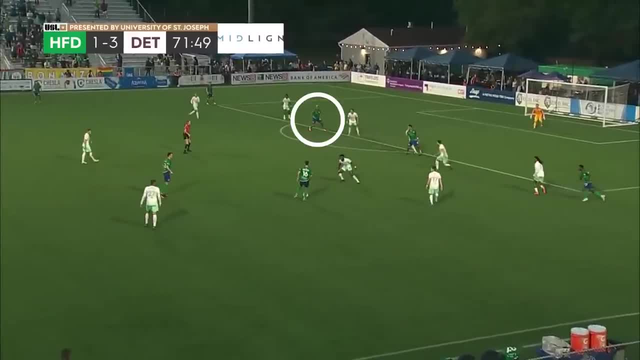 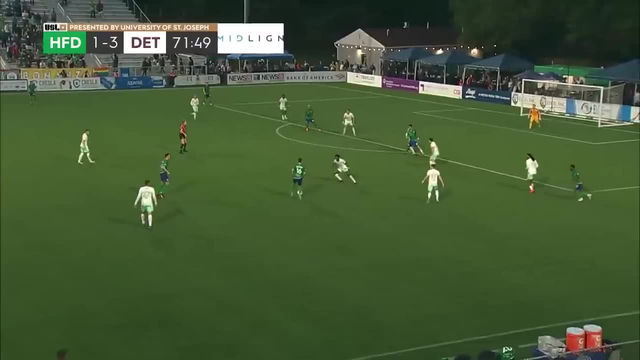 opposite of what what's given to you. And as I drive inside, Kyle Edwards now is going to make a great checking movement right into this space, right on top of the box. So I was going to play Kyle right to his feet, to his right foot, And uh, he does a good job. just to keep that ball. 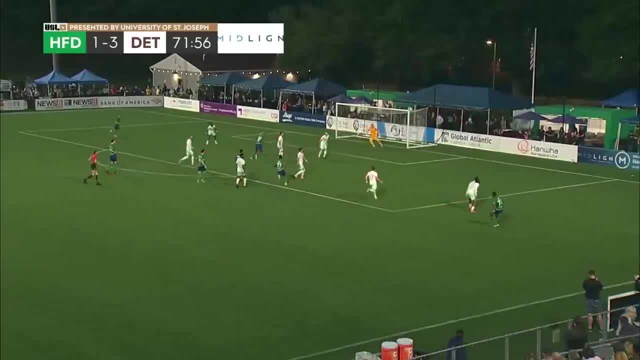 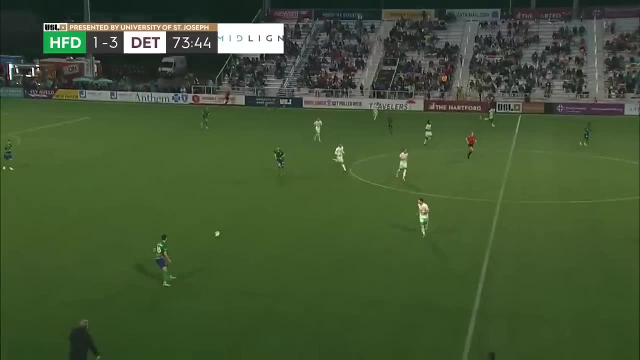 Back into Andre, out wide to Rideau and just get in the box. Now this is a good ball from Rideau towards the back post. Now next play, 74th minute, ball comes into Connor. I'm just going to get high and wide to receive this ball And then now, looking at this winger, kind of more of an inside. 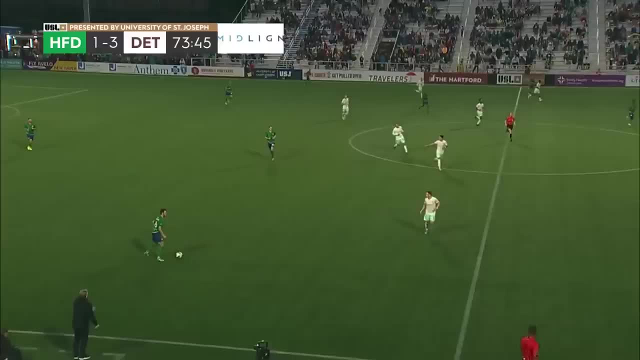 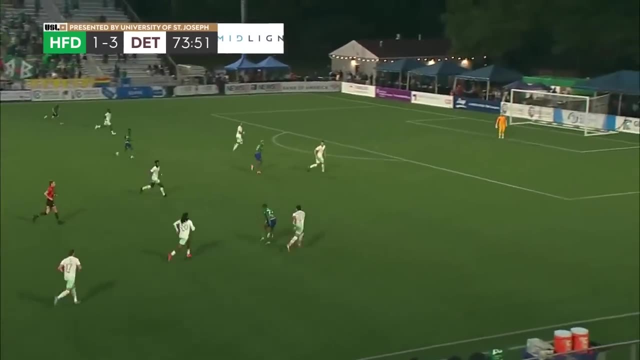 position kind of forcing me wide. So I'm going to do exactly the opposite now and play down the line into Rideau, play right into Rideau's feet. He does a great job here, Great little nutmeg, and he's off. This is a great uh sequence from from from Rideau. there Now goal kick from Detroit. 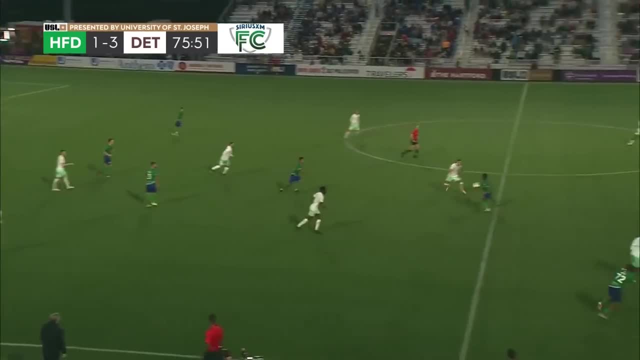 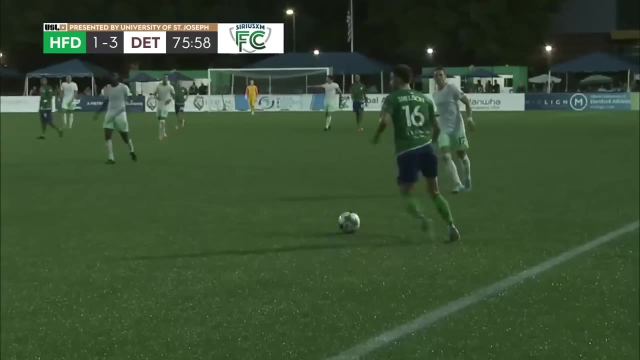 city bounces all the way back to me. I'm just heading this up the field and into one of my center mids, JP who comes and finds Andre who plays me back. It's a little bit out wide So I'm just going to take my touch forward, look forward And then, when it's not on playback, to. 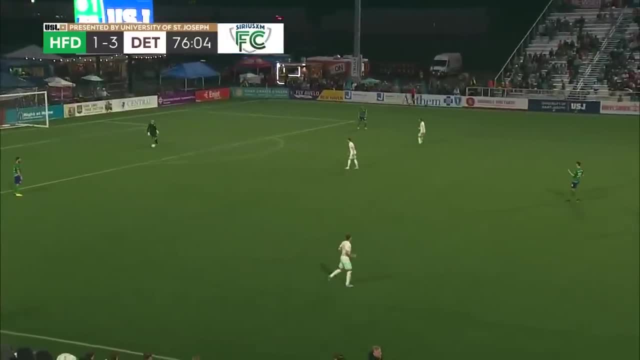 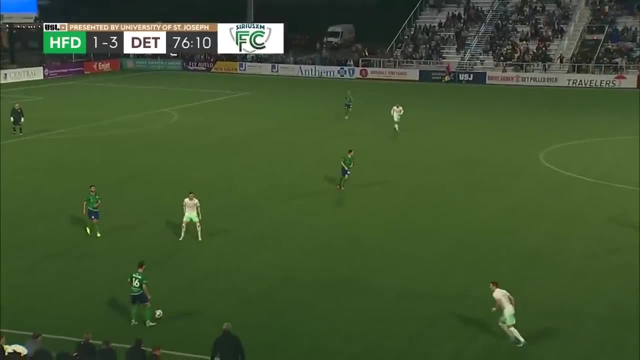 Joe rice, so he can switch it over to this to this opposite side if he wants to. Um, and again, just getting high wide waiting to receive this pass as it comes again opening up, once again watching the winger. he's cutting off the line now, which means we go in towards the center of. 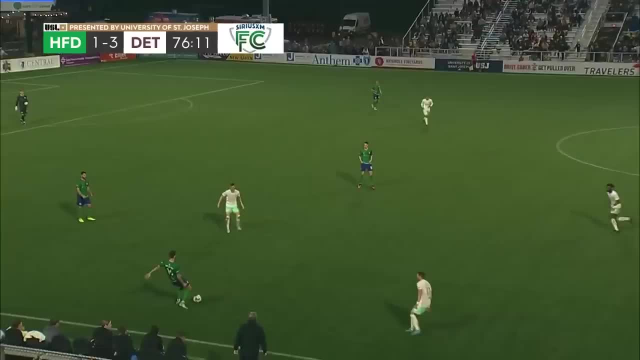 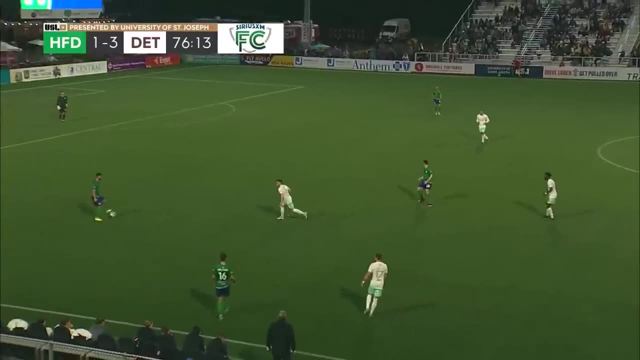 the field. Connor's checking his shoulder. He's ready for this. So as I'm about to play Connor now I start to see this player and this player start to make moves towards him. So I second guess myself, hold it and then just play back to my center back. Uh, just wasn't ready, Just was a second. 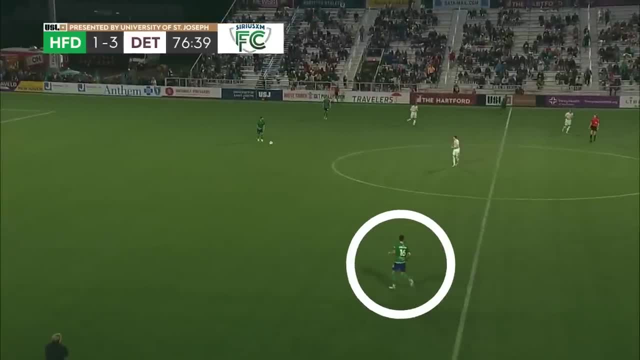 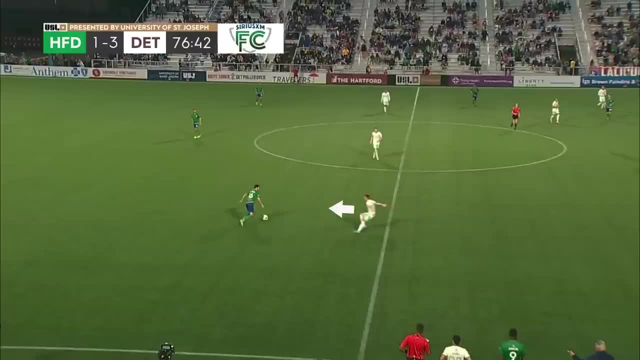 light to play that And they read that, So I just wanted to be safe there and play it all the way back, Um, receiving this ball from Kaveh, checking my shoulder a couple of times for that pressure- I know I have a lot of pressure- And then again just taking a touch in the opposite direction of 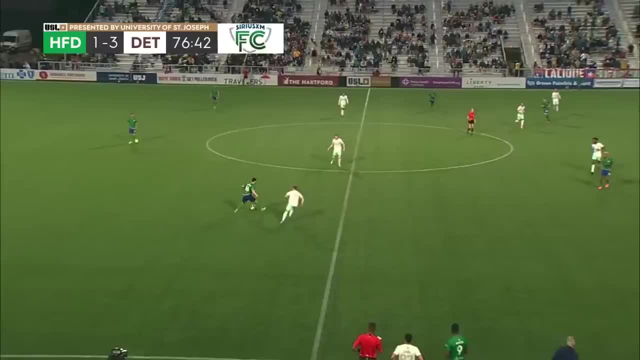 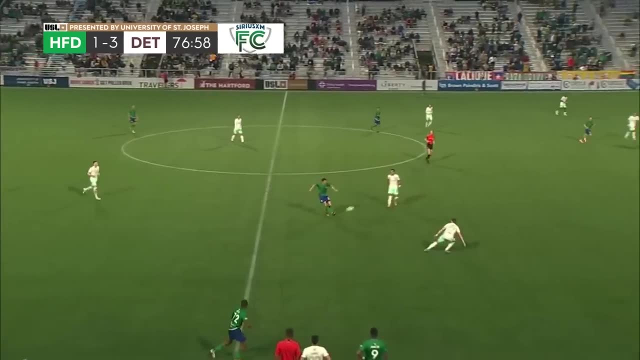 the momentum. So the winger comes in, he starts to uh touch, starts to fly out, has to slow down, pause. I take my touch inside and then just play it back and continue my run inside into this, this area. Now, this is a great ball from Connor riding. 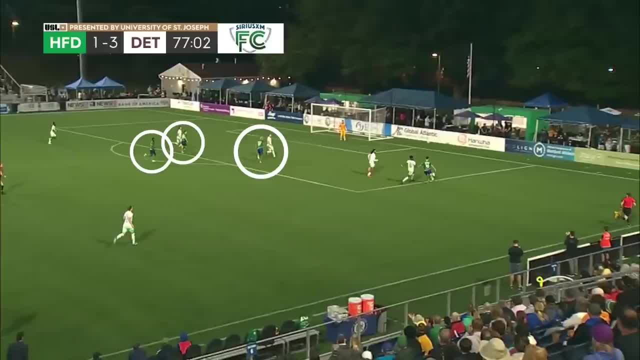 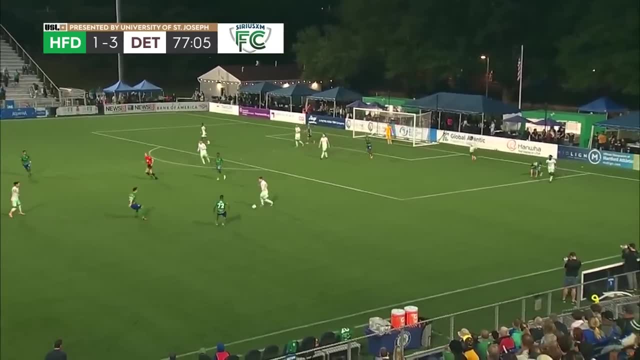 behind, right on the side of the 18.. As it comes over, I know I have three players in the box just out of my peripherals, So I'm just going to try to play this ball hard on the ground into the box. Um, and just goes right into Carol. there, uh, the guy right on the front post. 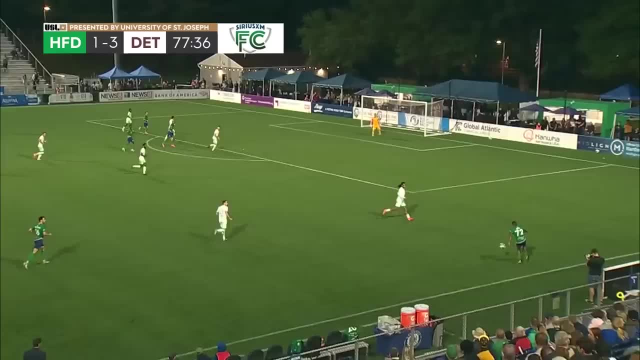 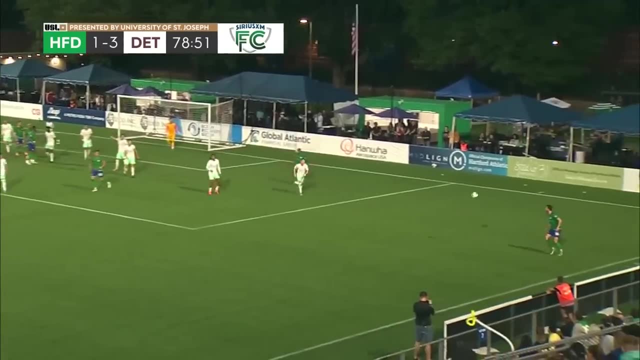 receiving the ball. Now, turning looking forward, real has got tons of time and space to take on their left wing back one V one. So I'm just going to play this ball hard on the ground and just play that ball pretty quickly into him. Long throw into the box is going to come right back. 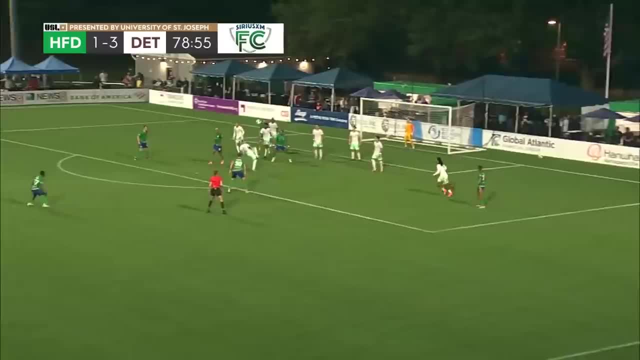 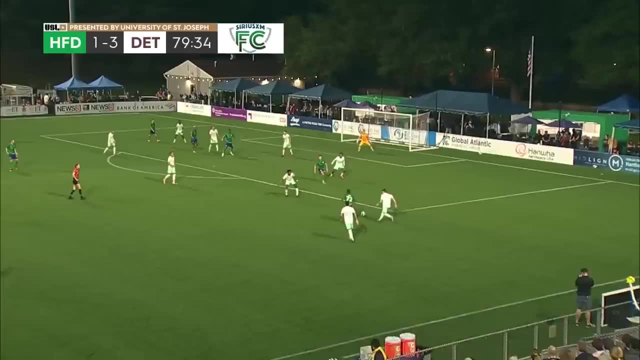 down to me. I'm just going to play that ball on my right foot and try to hook in across into the box. Um, unfortunately I don't find one of my teammates, Rito one V one and the side of the field here just popping into this space. uh, on the different pages I've wanted the ball to. 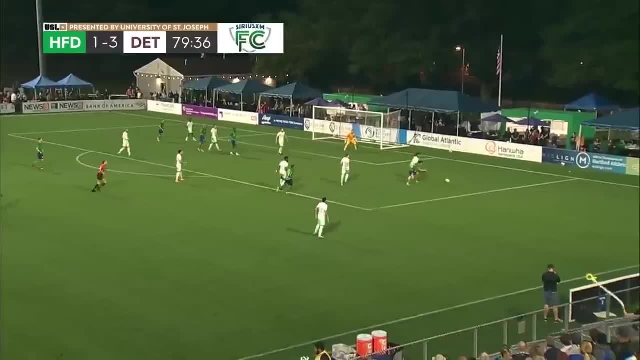 feed just popping into space. Rito plays this ball in behind. It's a good ball. just a little bit It was. I wasn't ready for it And, uh, I take my touch and it goes out of bounds, but it's. 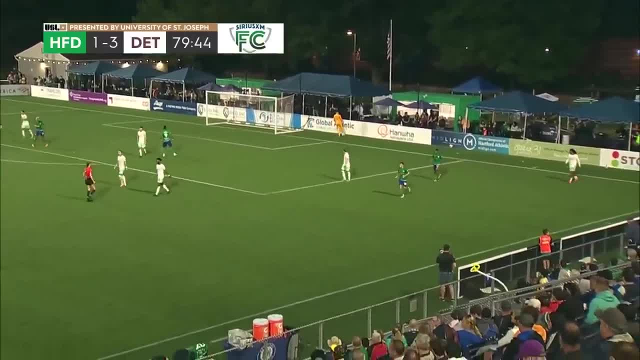 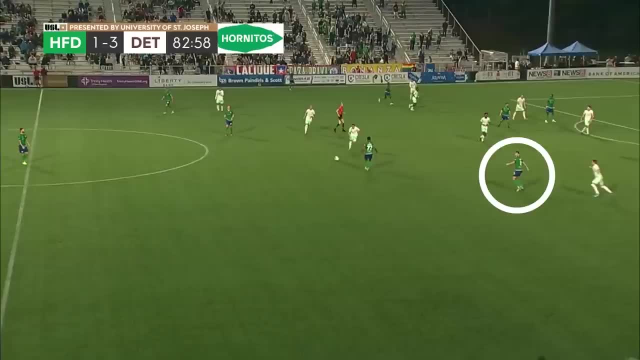 a good idea from Rito. It is, I think, the first time that we're playing together as him. as a winger, he has a right back, So we just have to start to learn each other's tendencies like that. Now, here I'm just checking my shoulder to see where Rito is, my winger. 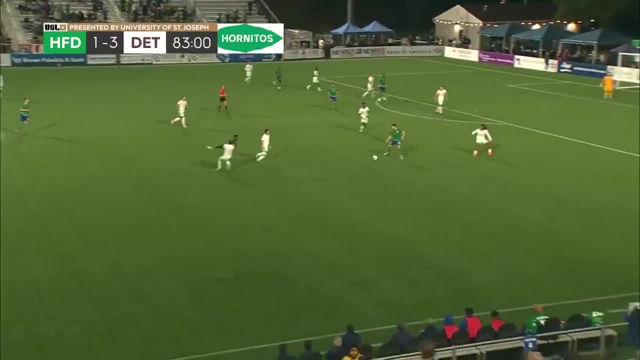 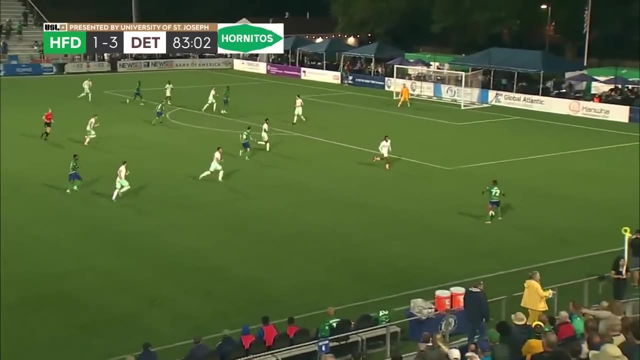 So I can. I want to stay inside, so he can stay outside. Andre, with a great slip pass, And now I don't even have to look, I know that he's wide open out here. One touch, without even looking at, can just play this ball out to him and he can whip in a great ball. This is a great cross. 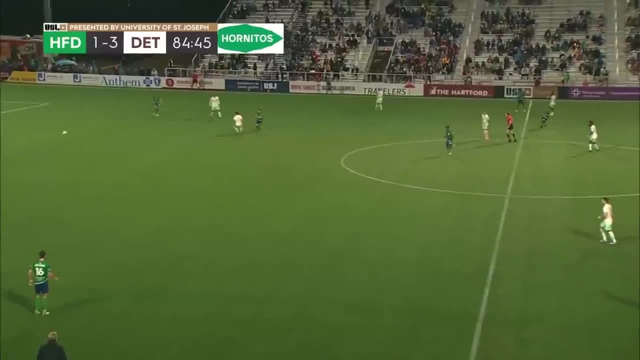 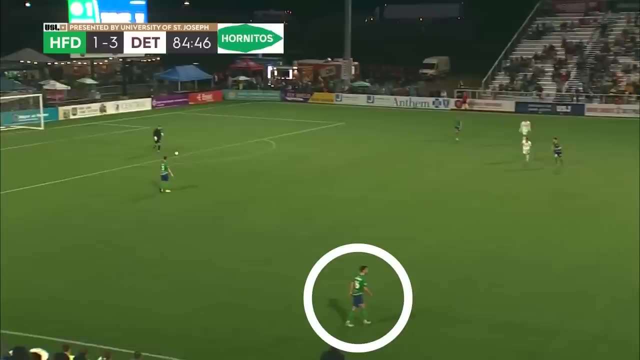 into the box there And unfortunately Elvis isn't able to get on that, or I think he might've glanced that header. but great ball from Rito. Now here's a movement That you'll see a lot um from many different teams as a right back I'm just going to make 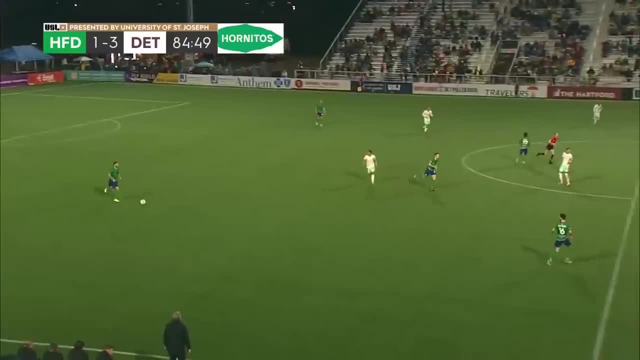 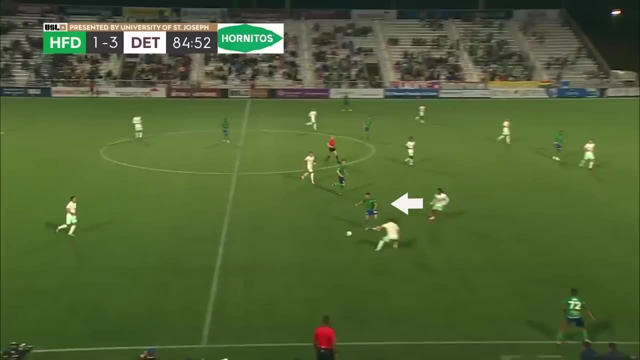 my run inside So Rito can drop, my right winger can drop and receive that defeat. So you can see I'm making my run inside and then he can play me. And as soon as he plays me in here- now look at Rito- He's wide open, Cause this forces this left wing back now to step to me, So now I can just 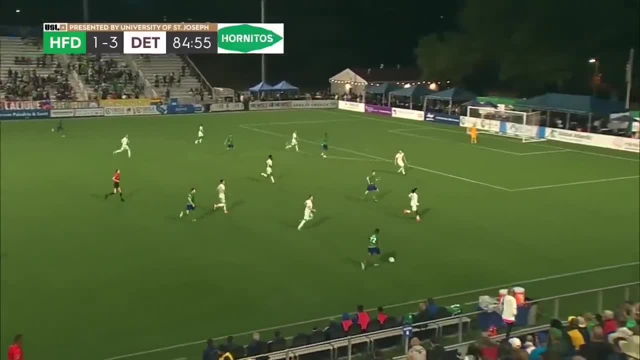 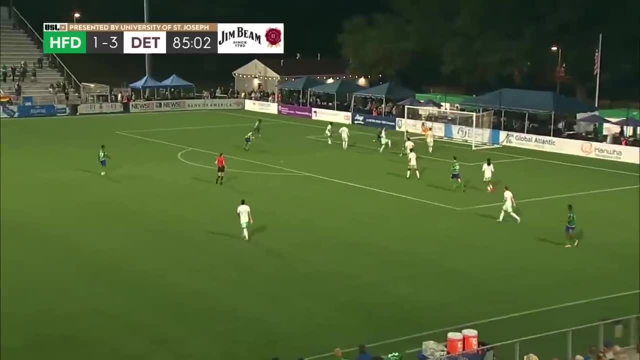 open up my body with the left foot, play right into Rito. It's a little bit slow, Um, but this is a good. again another really good attacking sequence down this, this right side from Rito. and another really really good ball. Another great, great cross from Rito. 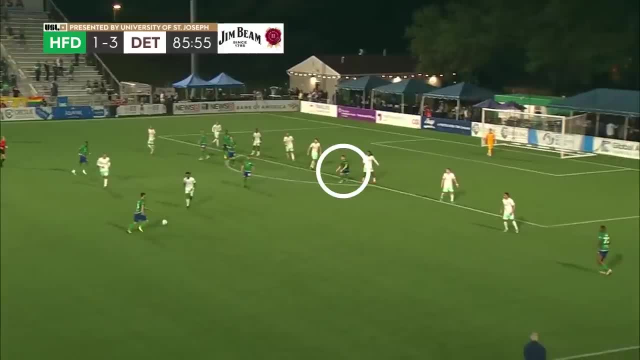 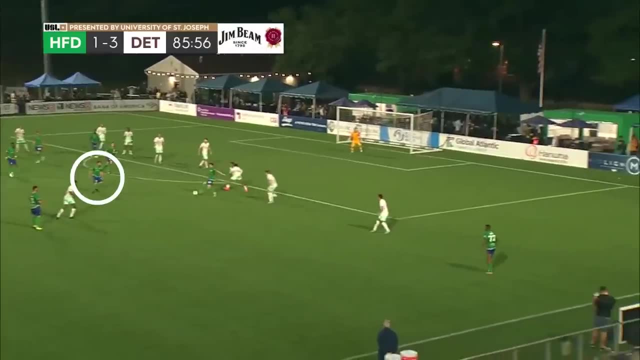 Rito, our right winger. Now I'm just right here, center of the field. You can see Detroit city's really packing in here, as they should. five minutes left to go in this game, receiving this ball, and Danny's in a really good spot. So I'm just going to one touch it. since my 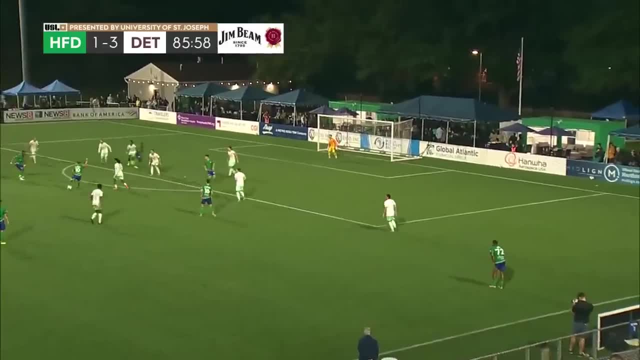 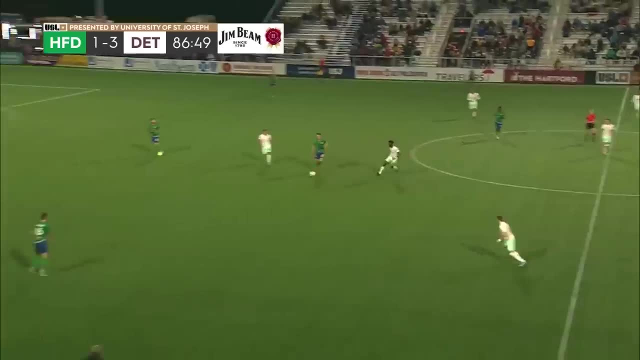 back's to goal. one touch to Danny and hopefully he can get a shot off. And, uh, he does this a great little move to his right foot and tries to hit it to that far post. It was a good shot from, uh, from Danny Barrera, Now receiving this ball from. 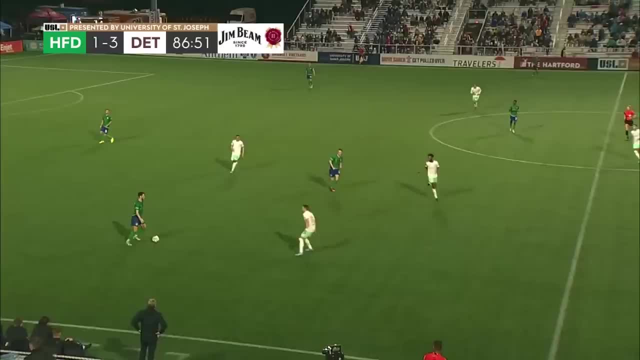 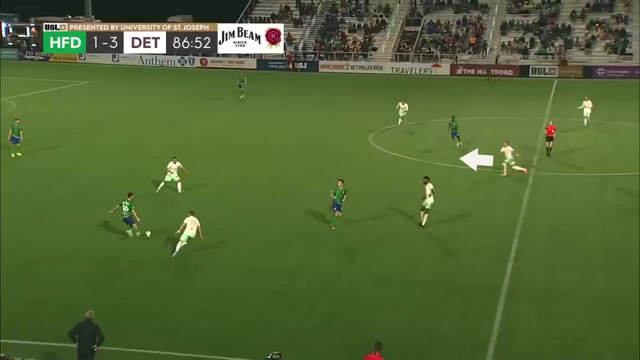 Connor starting to get some pressure in here. Uh, once again he's kind of cutting off the line. So I'm going to look centrally, take my touch centrally. I don't think this passes on. I think it's well read. I think this is Maxi Rodriguez, So I'm just going to play. 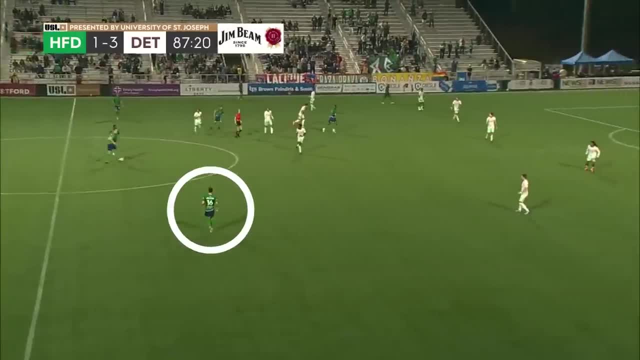 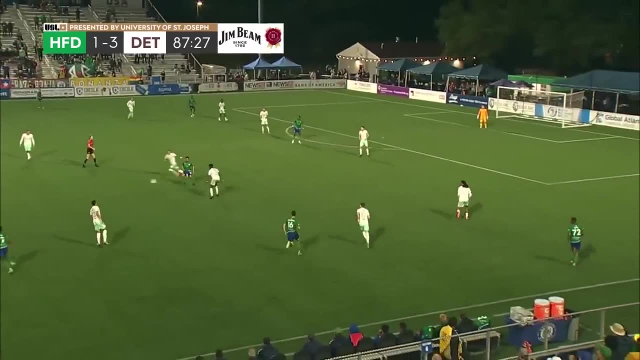 it all the way back to Kaveh. Now, who can swing it over to the opposite side, checking my shoulder once, twice, three times, receiving that pass And then just playing right into Andre Lewis's feet, as he's calling for it, And then again making my run inside up the. 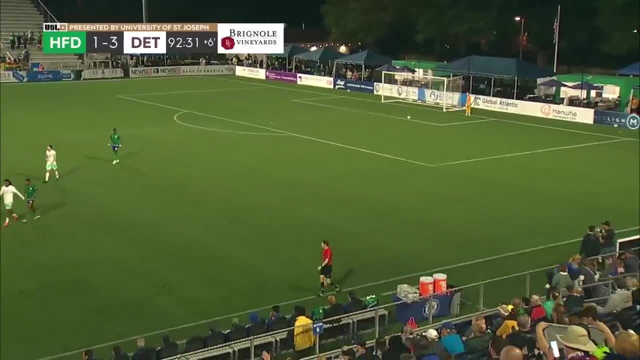 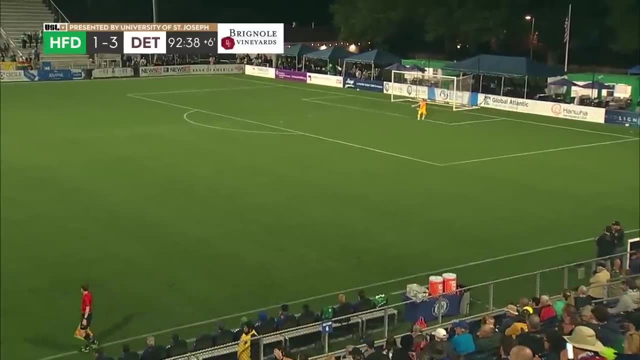 field trying to get involved in the attack. Now, 93rd minute, Now time starting to click. uh, tick down Detroit city FC with the goal. kick Steinwasher, Yeah, Clears it up the field. And then here is a foul for me. I thought that was really, really. 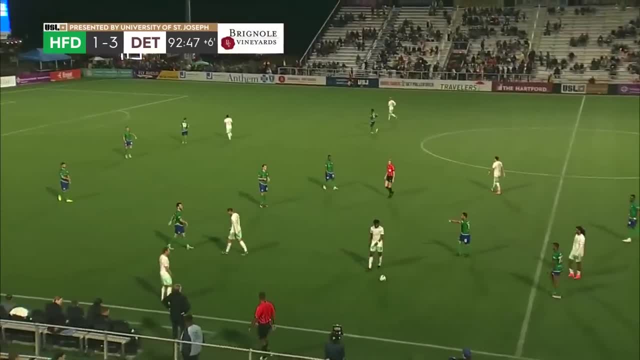 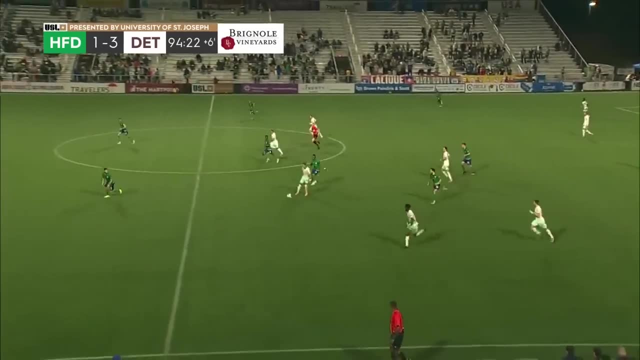 soft. I was just on the back of of this player And uh referee calls me for a foul, said I was uh holding him. And then, last couple of minutes of the game, counter-attack from Detroit city just working my way backwards. Now you know they're going to go straight. 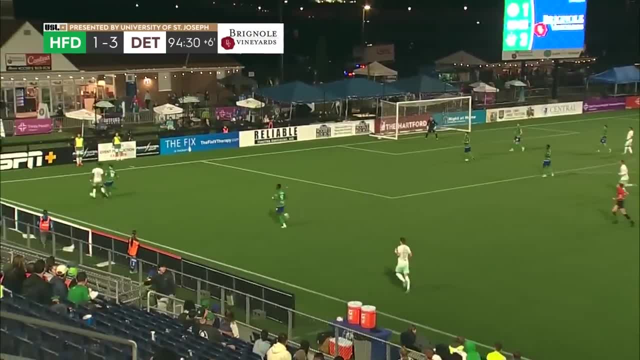 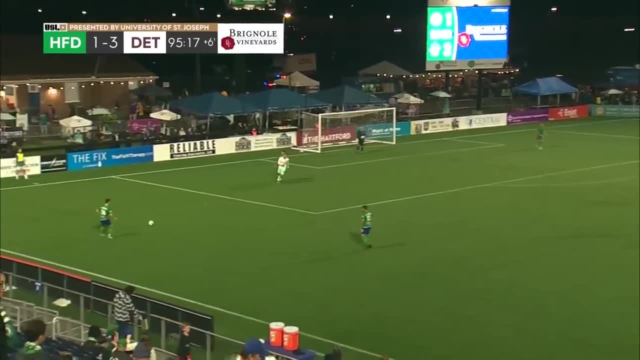 to the corner flag and try to delay, try to waste some time here. So I'm trying to kick this ball off of a Detroit city FC player And unfortunately it ends up still being their ball. Now, ball to me last minute or two. just give it to my center mid, have him create something. 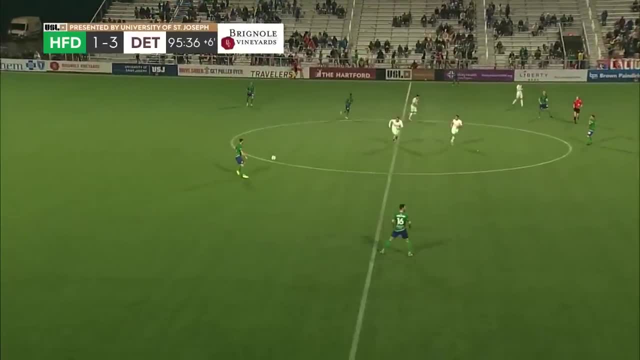 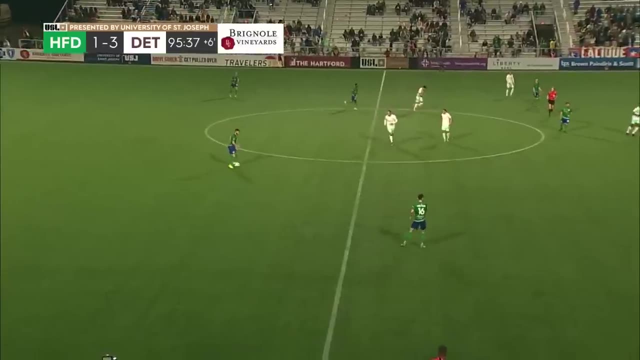 and push up the field And then this is like the last play of the game. I have tons of time and space and this is just. it's not a good play. tired legs and tired mind and frustrated mind, but I'm going to receive the ball. a couple of shoulder checks, I know. 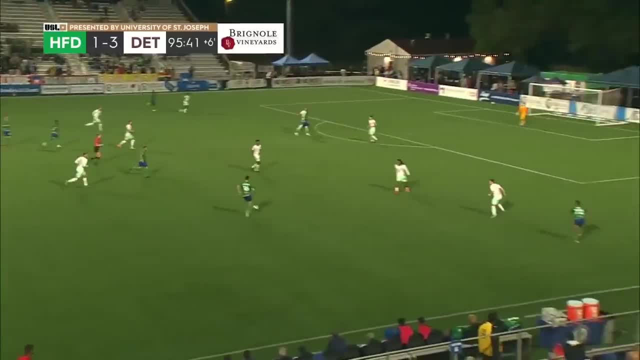 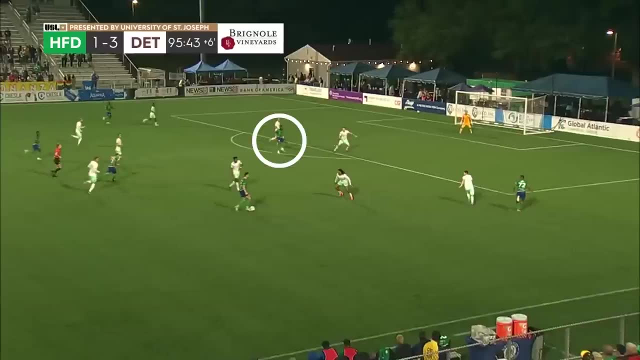 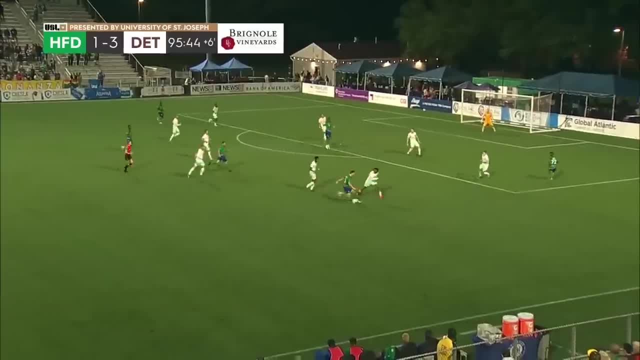 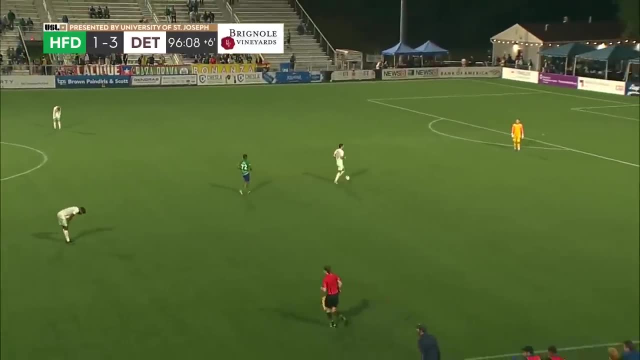 looking for Rito now and I can't find a passing lane to play in Rito and behind. And then I kind of get myself into a pickle here, take too many touches and then lose the ball, So wasted opportunity. at the end I'm a little frustrated with that play, but I think overall 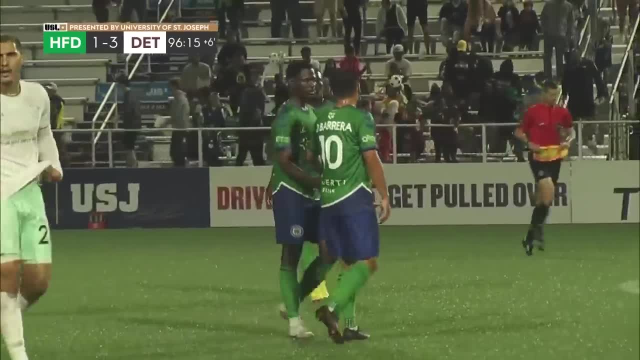 I think both as a center mid and that first half I think a pretty good game And I think in the second half as a right back, I thought it was pretty sharp. you know, I'm obviously gonna have one or two plays where it doesn't work out. 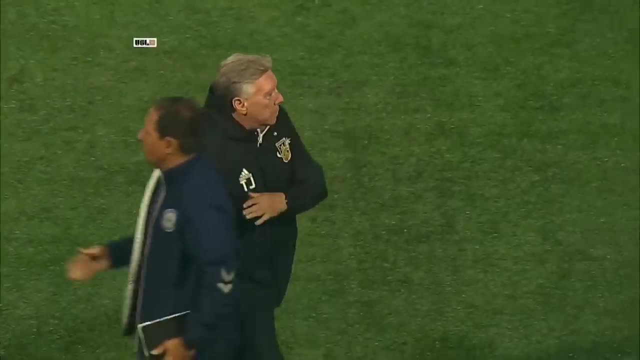 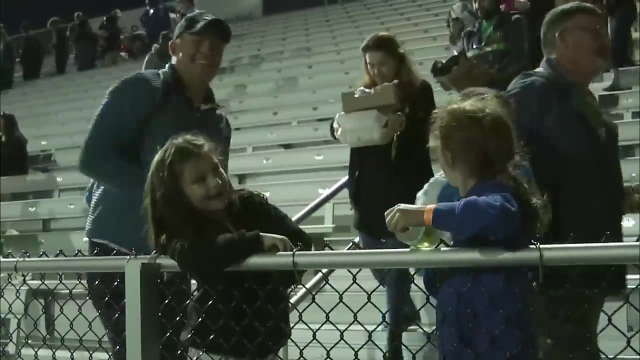 But unfortunately for us, we lose this game. Three: one um Um, Detroit City had a good game. I thought they created some great attacks, uh, and even with the penalty save, you know, they could have been up, easily been up 4-1 from us. so tough game another.